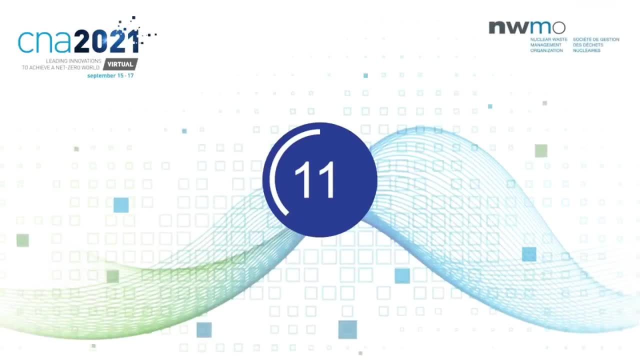 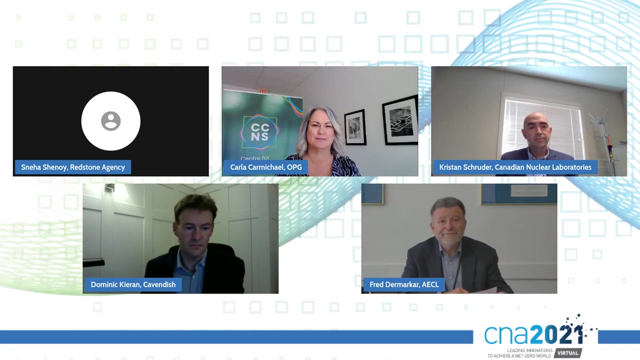 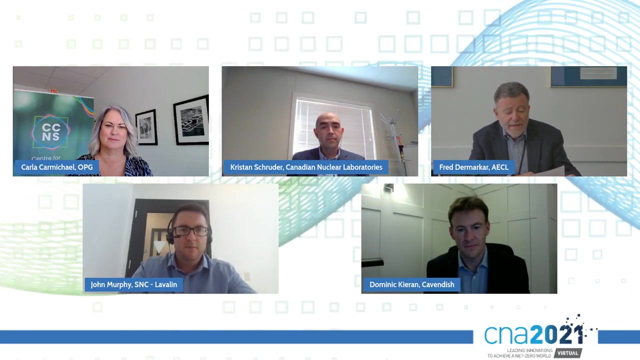 My name is Fred Remarker and I'm the President and CEO of AECL, and I'm talking with you this afternoon from the Chalk River campus of Canadian Nuclear Labs on the traditional lands of the Anishinaabe and Algonquin peoples. We have a great panel this afternoon with representatives. 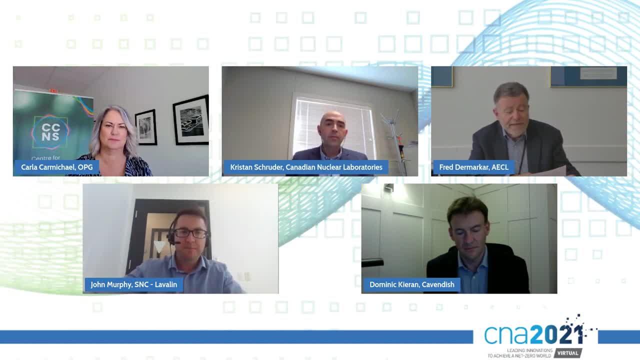 from Ontario Power Generation, Canadian Nuclear Labs, Cavendish Nuclear and SNC-Lavalin, And before I turn to them for remarks, I'd like to set the stage a little bit First. when we talk about decommissioning, we can't lose sight that we are talking about facilities that have contributed. 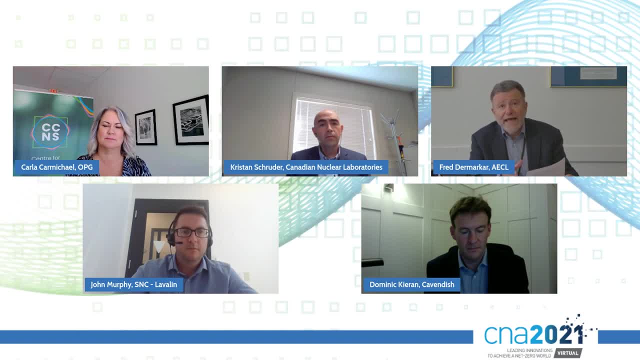 tremendously to the nuclear community in Canada and around the world And, just to name a few, science and technology labs that have advanced our knowledge and positioned Canada as a well-respected leader in the nuclear field. And it's notable that two of Canada's Nobel laureates were 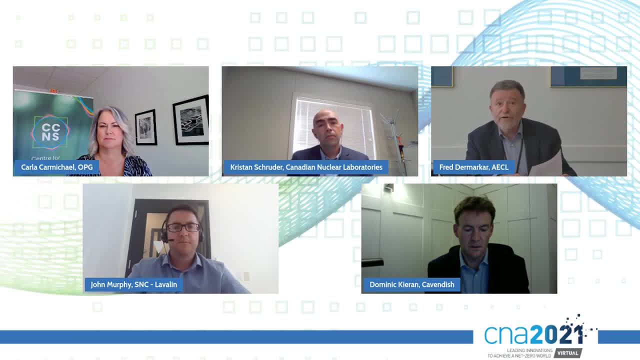 got started right here at Canadian Nuclear Labs and did a lot of their work: Demonstration and prototype reactors that have enabled us to develop can-do technology, which accounts for more than 10% of power reactors around the world. Nuclear utilities that produce 15% of electricity in Canada. all carbon-free And medical isotopes that have contributed to 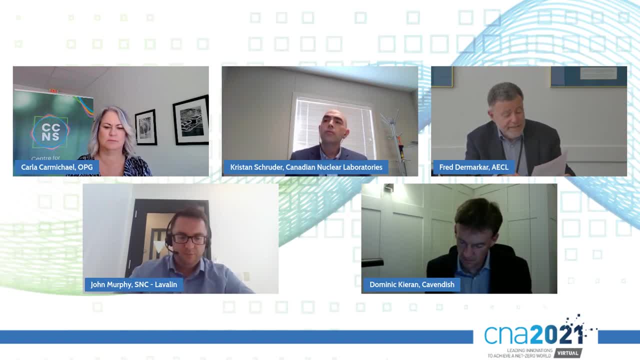 more than a billion diagnostic tests and procedures, improving the lives of Canadians and people around the world, And I'd like to start by saying thank you to all of you for joining us today. This is an important part of the story behind decommissioning and we have to 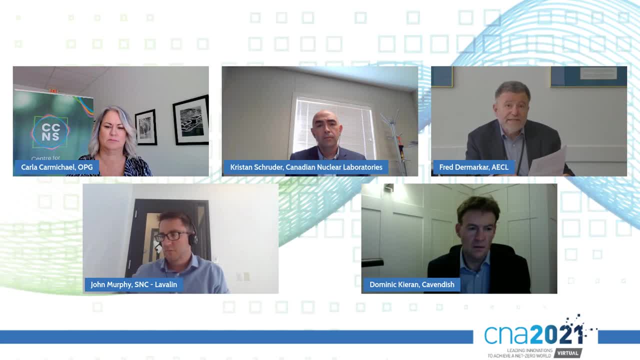 keep repeating it Now, most of the facilities that we are decommissioning have played a significant role in nuclear innovation, so it makes sense to look at innovative ways to decommission them. Importantly, innovation and decommissioning doesn't just mean robotics and other state-of-the-art. 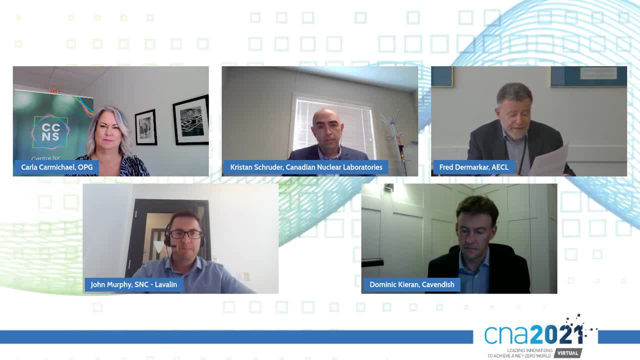 equipment. Innovation is also about new ways of working together. It's about collaboration in the supply chain. It's about bringing together the people that are in the supply chain. It's about bringing together the people that are in the supply chain. It's about bringing together the 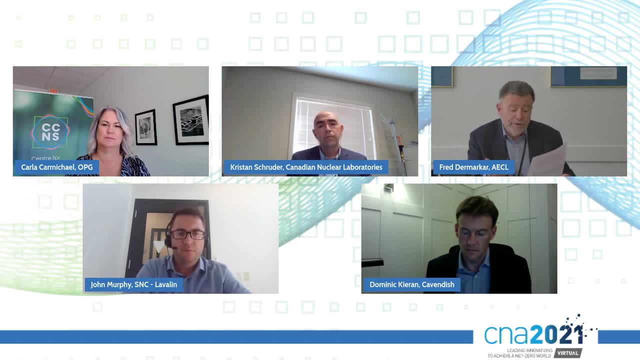 right expertise, going beyond our nuclear community and embracing innovations developed by other fields. And it's about working with Indigenous communities. It's also about bringing to bear our collective experience and capabilities and leveraging them for increased commercial opportunities abroad. Canada has always punched above its weight when it comes to nuclear. 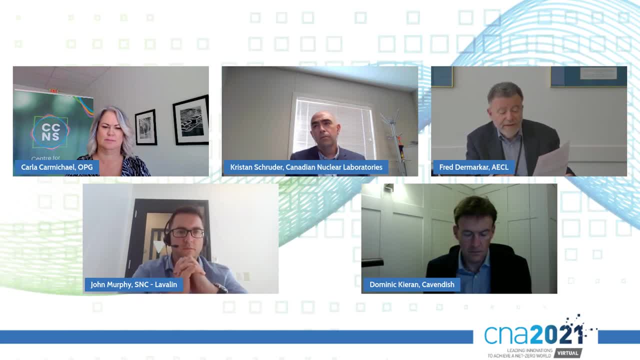 and we will continue to punch above our weight by continuing to take a team Canada type of approach, as we have done in the past. Nuclear decommissioning is an enormous and growing market, So how do we innovate here and abroad? The people here today have the expertise. 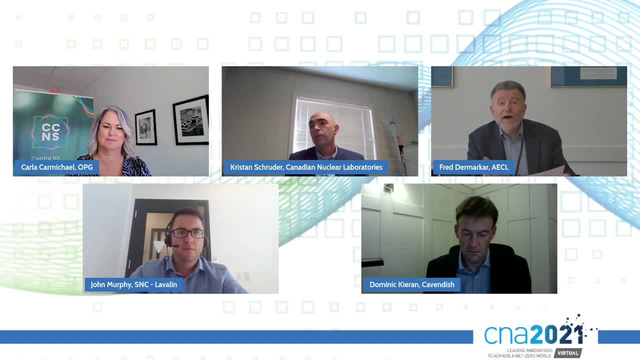 and will be sharing with us their perspectives on how we will do this. So I will turn it over to them, And I'd like to start with Carla Carmichael. Carla is the Vice President for Decommissioning Strategies at OPG. Thank you, Fred, Thank you for having me and having this opportunity to talk about decommissioning. 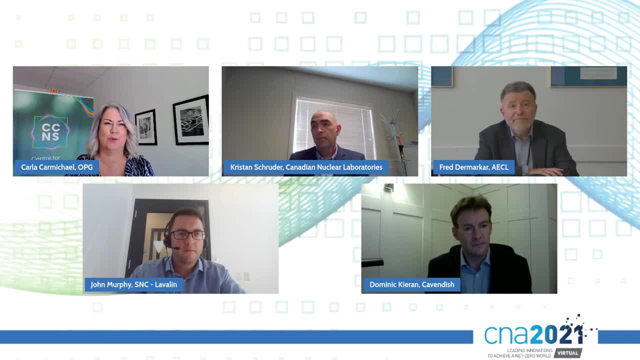 Decommissioning a nuclear plant, as we know, is a very long-term, complex project, In particular our eight reactor unit facility at Pickering Nuclear Generation Station, which is going to be a first of a kind Decommissioning project and have a lot of different scopes of work and also challenging. 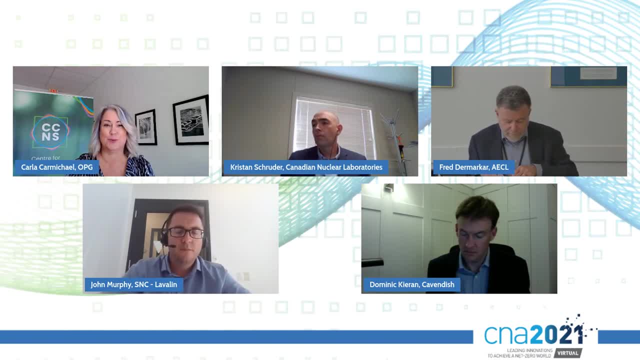 because of its proximity to Toronto. So we're looking forward to that challenge. What we are doing at OPG is to support the planning and eventual execution of this complex mega project. is OPG's launch the Centre for Canadian Nuclear Sustainability, or, as I call it, CCNS? 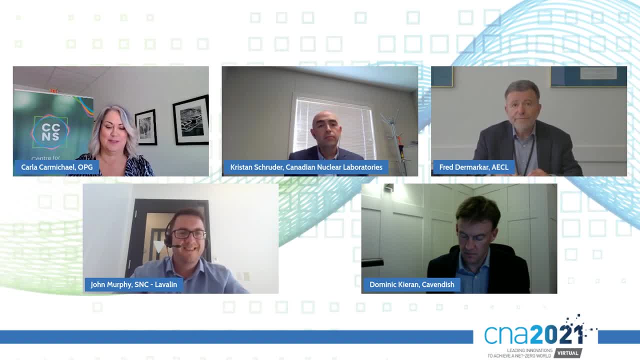 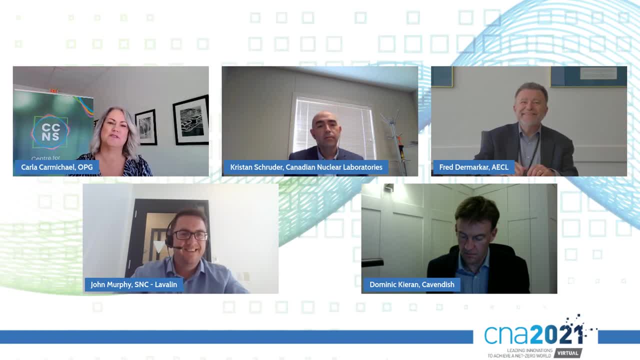 the CNSC. okay, The Centre's goal is to facilitate and demonstrate that we are building tomorrow together by mobilizing research and development and collaboration to advance innovative technologies and opportunities. that really bear on some of that: those toughest challenges in nuclear decommissioning, waste stewardship and site repurposing. And I think, as Romina mentioned, 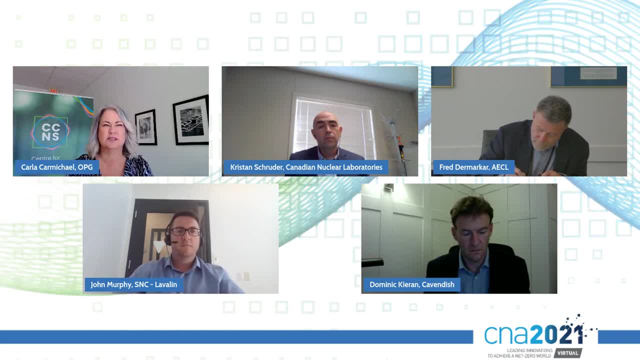 fell she mentioned at the last session. it is sort of seen as achilles heel of the industry. the ccns is located in pickering and is attracting skilled jobs, innovative businesses and economic development to the durham region. our partners are made up of industry organizations and associations. 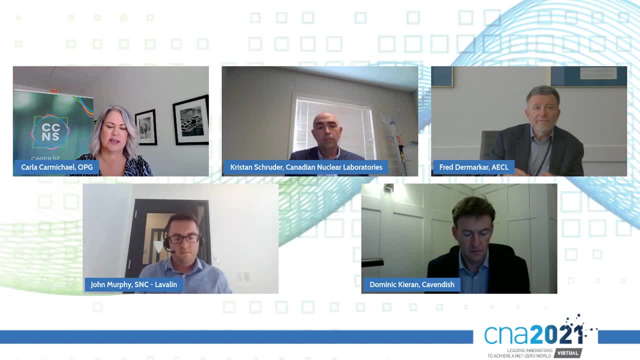 academia, local businesses, indigenous communities and, on our host communities through the center's collaboration model, which has been set up. the vision is that nuclear remains a sustainable energy source for future generations. to ensure a clean energy future for generations to come, the center launched what we call an innovation fund: not designed, designed to not be hindered by 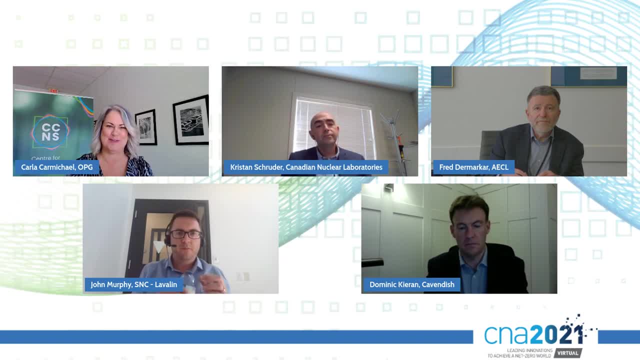 typical bureaucratic processes that sometimes we've faced in our past and also not hindered by sort of these corporate roi hurdles that we also had to overcome. the focus on these investments is really to prepare for decommissioning and advanced solutions that will reduce the timelines costs of these decommissioning. 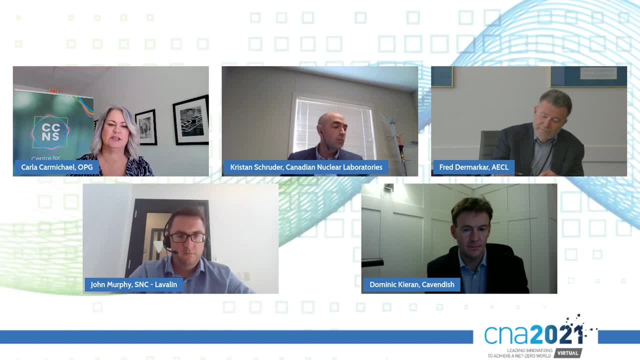 projects and enhance employee safety, reduce radiation exposure and waste and ensure that safety for the community environment. so i'm really pleased that the other participants on this panel are all partners of the ccnf and have been working with opg and with each other to solve these challenges. opg knows that we can't 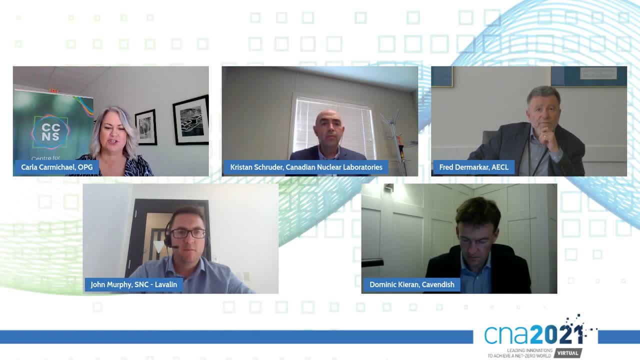 do this project alone and that we need innovation, that the industry and our communities have to be part of this solution. decommissioning a nuclear plant is complex, like i said, and will be very challenging. it's not enough for our industry to have strong nuclear operations and refurbishment. 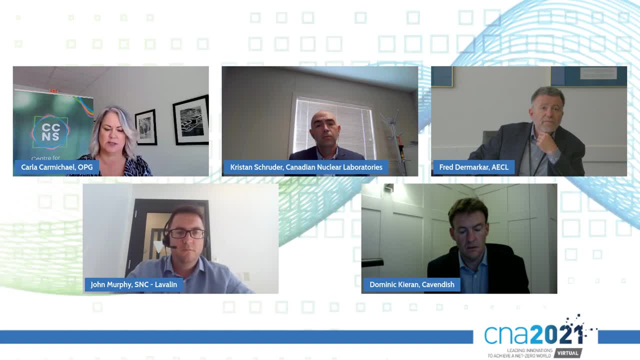 performances to maintain our social licenses. we also need to demonstrate strong end-of-life management of our nuclear assets. demonstrating success in all aspects of the nuclear life cycle enables us to grow the industry, which we all know is vital to achieving this net zero world that we want to achieve. to support the planning and um and. 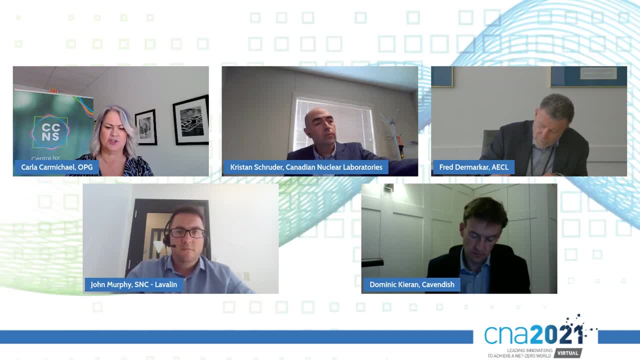 eventual decommissioning of it. i'm very happy to say that we've joined forces to do that and and look forward to working with you all in the future and and look forward to hearing what everybody else has to say. thank you, thank you very much for that, carla i. i. i love the tagline: building tomorrow together. 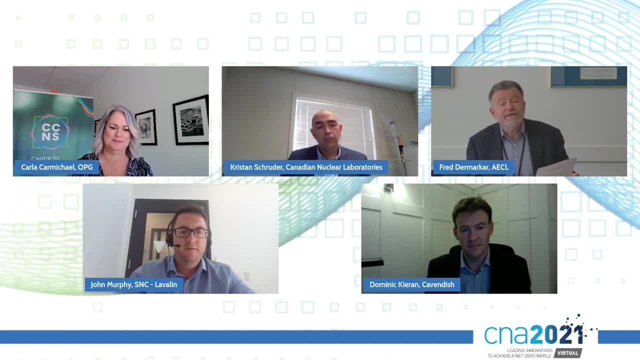 so next we're going to move to kristen schruder. kristen is the general manager and deputy vice president environmental remediation management at canadian nuclear labs. over to you, kristen. thank you, fred. i wanted to thank the cna for inviting me to speak on this panel and i'm 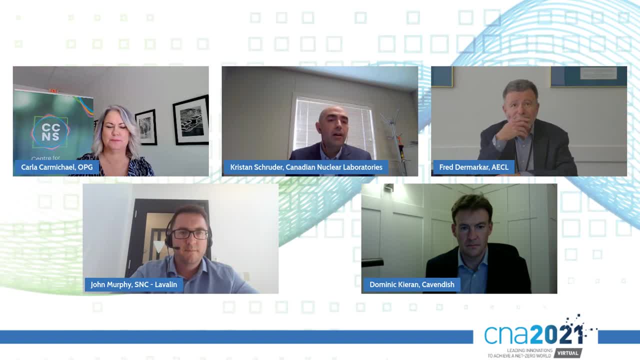 honored to be on this panel with such distinguished speakers. uh, i'm going to focus my opening remarks on the decommissioning work being undertaken by cnl in canada. for more than seven years, cnl- formerly acl- has been on the forefront of development of the nuclear industry in canada. 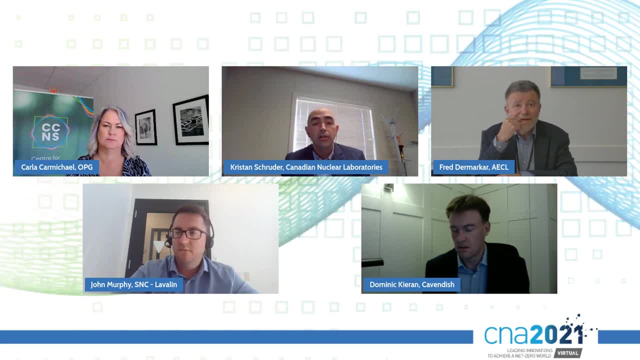 and today cnl is actively restoring and protecting canada's environment by effectively and efficiently managing acl's nuclear nuclear liabilities at multiple sites across canada. many of you may not be aware of the scale of decommissioning waste management activities currently being undertaken in canada. cnl has, on average, 1600 staff actively supporting 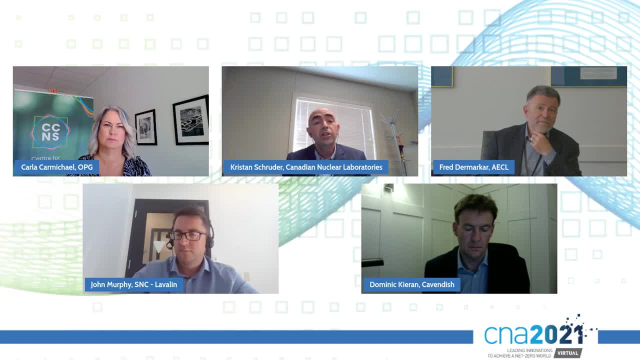 decommissioning and waste management activities at our sites. our budget this year is approximately 800 million and we're executing cleanup projects across eight sites. we've seen a dramatic increase in the cleanup efforts in the last six years with the implementation of the goco model. i'm 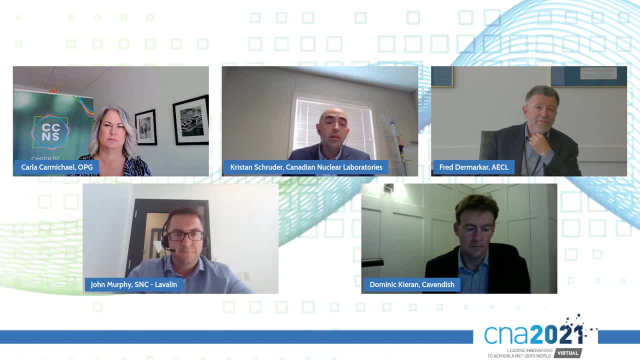 going to spend a couple minutes highlighting some of this work from a decommissioning standpoint. over the last six years, we've decommissioned over 150 buildings across our portfolio, which has resulted in a footprint reduction of approximately 450 000 square feet. we do everything we can to minimize radioactive waste and for this work we generated 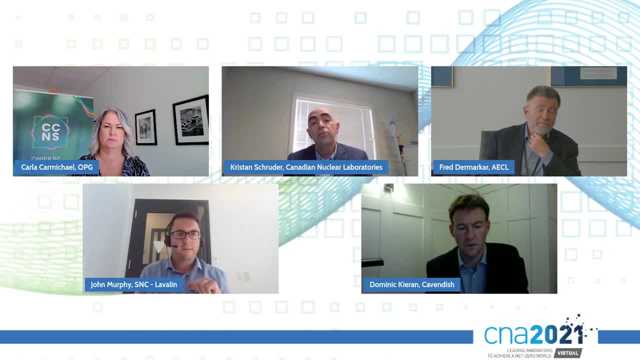 17 500 metric tons of clean waste, approximately 21 2100 metric tons of radioactive waste and 180 metric tons of hazardous waste, largely asbestos. there are three sites that largely contributed to this work: chalk river laboratories, white shell laboratories and devils point at truck river. we've taken down 105 structures since 2016, and this has largely been with our 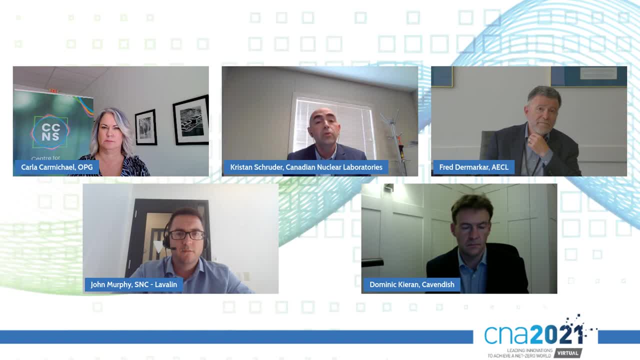 own workforce. we have approximately 500 staff supporting decommissioning work at chuck river. when the goku initially started, we had close to 100 staff supporting decommissioning and we've ramped up our team substantially to reduce these legacy liabilities at chuck river. at white shell. 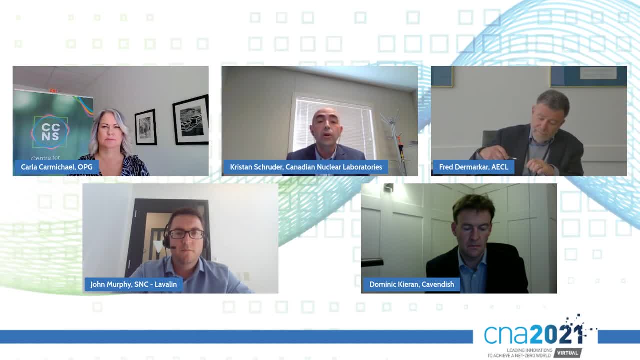 we're in the process of closing down this site. we completed operations at white show in the late 1990s and we've been progressing towards closure since then. at white show we've taken down over 35 over the last five years. we have a workforce of over 300 staff focused on the decommissioning waste. 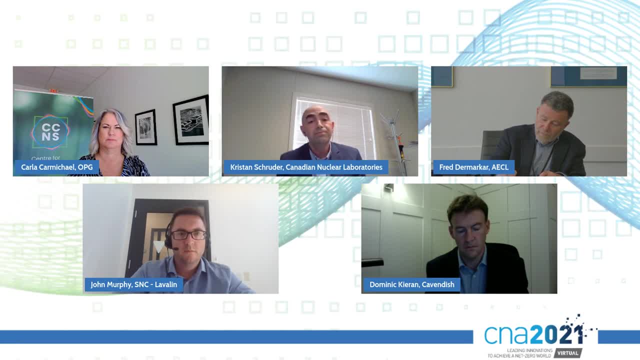 management activities in support of site closure, which is planned for 2027.. the third site where we have active decommissioning underway is at douglas point. we recently received cnc commission approval to transition transition this site from storage with surveillance to decommissioning. 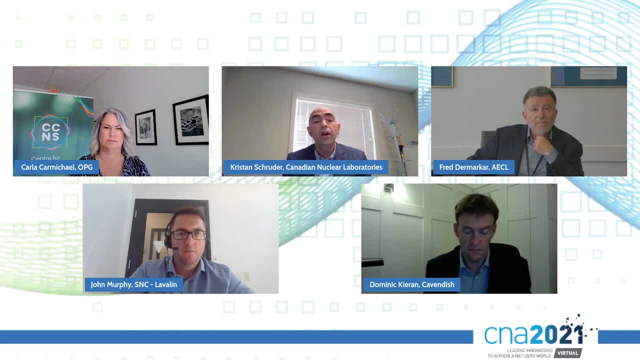 this will be an important project for canada because, although smaller in size, it is the prototype candy reactor from which the pickering reactors were based on. from an environmental standpoint, cno is leading one of the largest environmental cleanup projects in canada at the port hope and port granby sites. these communities were contaminated from the iridium processing. completed by elder out mines starting in the 1930s. we just recently completed the remediation of the port granby site, which resulted in the placement of over 1.3 million metric tons of waste into the long-term waste management facility that we built there at port hope we're in the 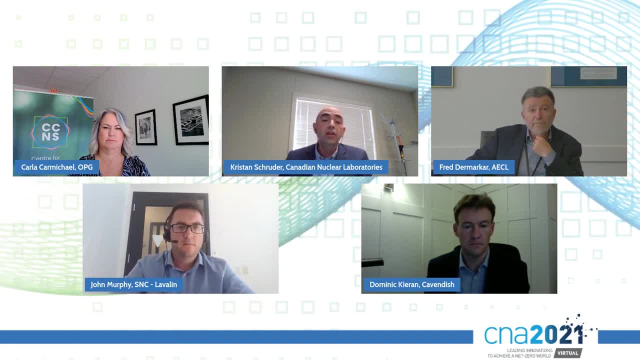 midst of remediation and have placed 1.2 million metric tons of waste so far into the long-term waste management facility and estimate that we have approximately 800 000 metric tons to go. this is a very complex project, as we are literally working in residents yards. 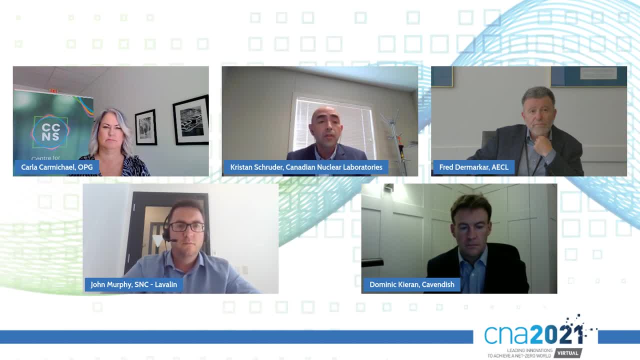 and even inside their homes, doing remediation work. from a waste management side, there's also been key achievements that i want to mention. it first has to do with fuel that we've been repatriating to the united states to support canada's non-proliferation objectives. canada- 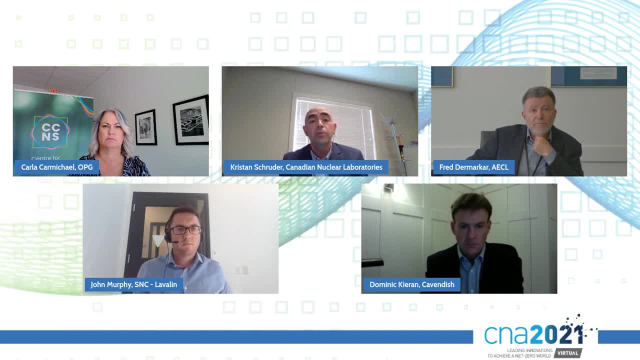 does not have a disposition pathway for large quantities of highly enriched uranium or heu cno. repatriated over 1 000 irradiated hd fuel assemblies from the nru and nrx reactors to the us in 2019, which permanently eliminated 120 000 tera becquerels of nuclear liabilities for canada. 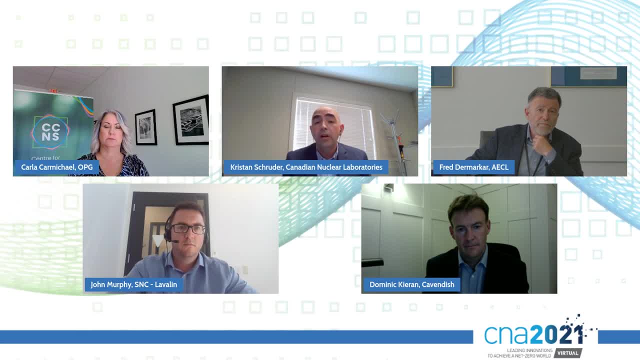 target residue material, or trm, was identified as the highest priority environmental challenge at the chalk river laboratories. the trm inventory included approximately 30 tons of highly enriched uranium nitrate liquid generated from medical isotopes, moly 99 processing. over the past couple years, approximately 22 000 liters of trm were recovered from a legacy waste tank and repatriated. 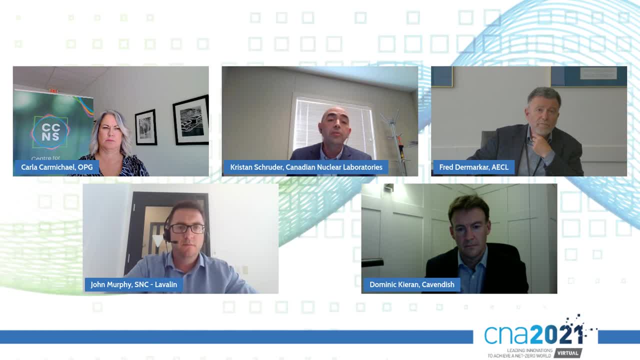 to the us department of energy. one of the key waste management projects underway at cnl right now is the near surface disposal facility. as you may have heard from my colleague, megan bicker, speak on this project at a panel this morning, cnl is planning to build low-level waste disposal. 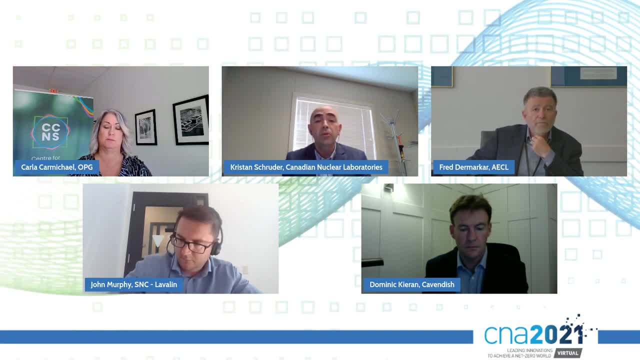 facility at our chalk river laboratories to safely manage and permanently dispose of low-level radioactive waste we are generating from our cleanup activities. this new facility will enable the cnc commissioning work and launch major environmental work at the chalk river site. we recently got acceptance from the cnc on our licensing and ea submissions and we're anxiously. 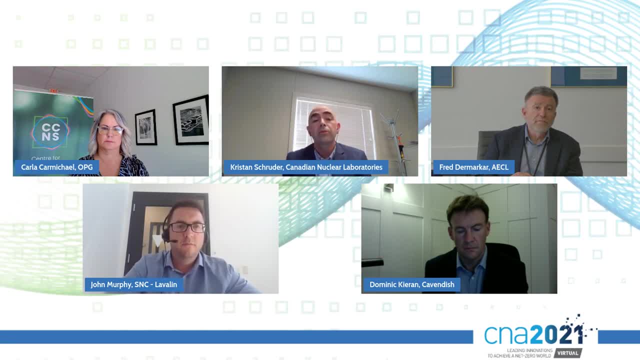 awaiting for the announcement from the cnc commission, hearing dates expected next spring. i think i'll leave my opening remarks here. thanks, fred. thanks very much, kristen. uh, a very impressive overview of the uh, the progress that's been made and- and i learned something new- today it sounds like 90 percent of 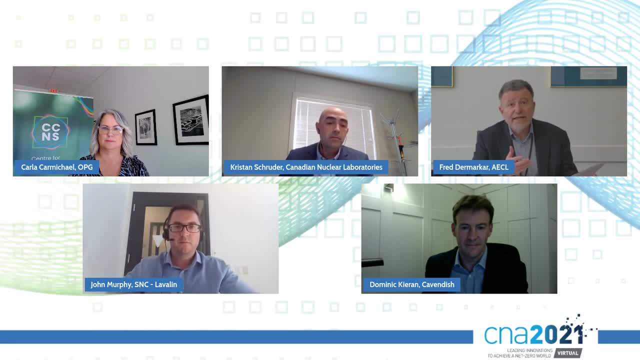 the waste that you generate, uh through decommissioning is actually clean waste and does not need to be disposed of, which uh, which is a good number to keep in mind. so thank you for that. next we have dominic kieran, who will share with us his perspectives. 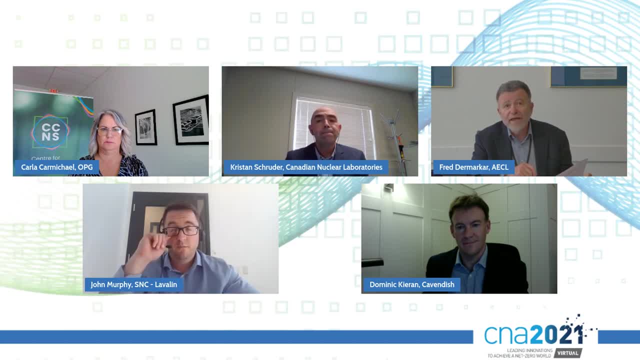 as the ceo of cavendish nuclear over to you, dominic fred, thank you and, uh, good afternoon everybody. uh, absolutely honored to be with you this afternoon. um, let me first of all maybe just talk about why do i think safer, faster, lower cost in the decommissioning area is important. 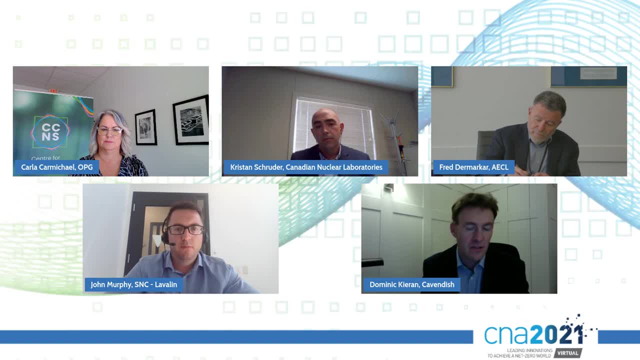 so i think what we're talking about here is us coming together as an industry to play our part in the decommissioning area, to show to our stakeholders that we, as an industry, can be trusted and can be trusted to deal with our legacy, and it's through that trust, then, that 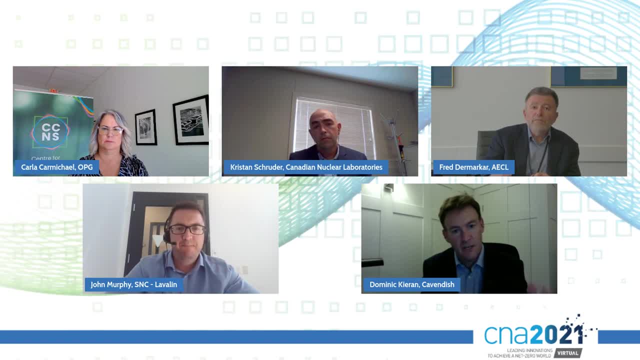 we want to be trusted to to take on the challenges of helping us transition to a net zero economy and, quite frankly, the huge role that i think actually nuclear has got to play in that transition. so i think we're, you know we're focusing here more on, uh, just sort of decommissioning. 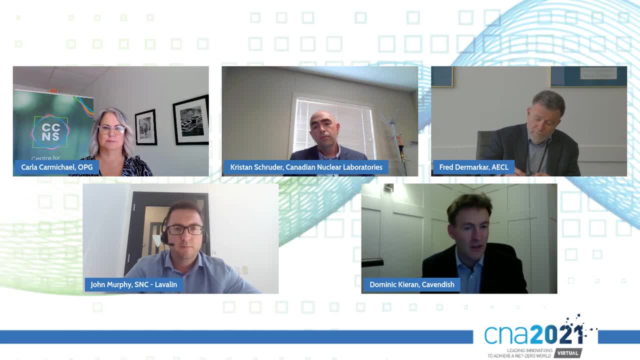 so with that sort of uh backdrop, maybe a a quick comment then about the sort of theme of the conference, which is uh sort of safer, faster, lower cost and innovation. so when we talk about innovation, a lot of people immediately sort of think products, products to help with uh, with sort. 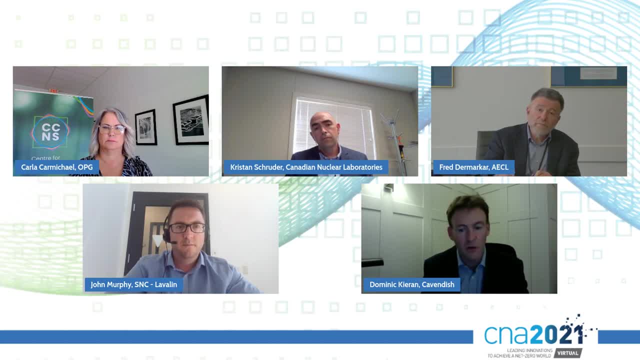 of decommissioning um- and they do have a very important role in that because they're very, very important role um- but i think what we see is that it's the sort of overall framework that you undertake decommissioning can can actually be more powerful. and i know, john, you're going to say a few. 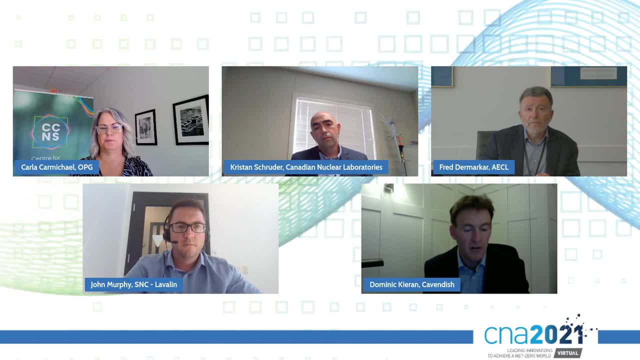 words about that as well in a minute. so our experience shows us that to enable the sort of safer, faster, lower cost areas like proportionate safety cases, waste treatment approaches and waste management really have a huge impact. and what's interesting is- i think this is particularly true- 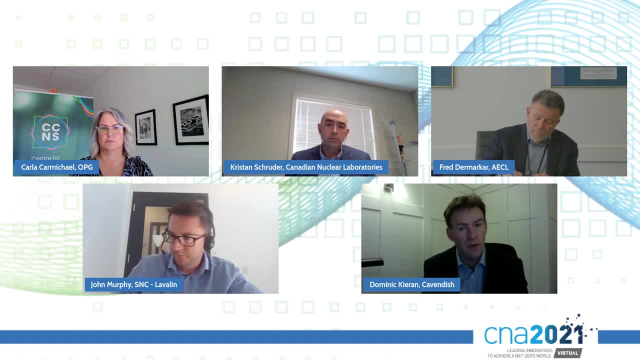 for a lot of the regulations, such as the uk and such as canada, where the regulator is less prescriptive- uh, and actually the the uh, the challenges for us as the industry to work with the regulator to prove that what we're doing is is safe in our lab. so, in that regard, i actually 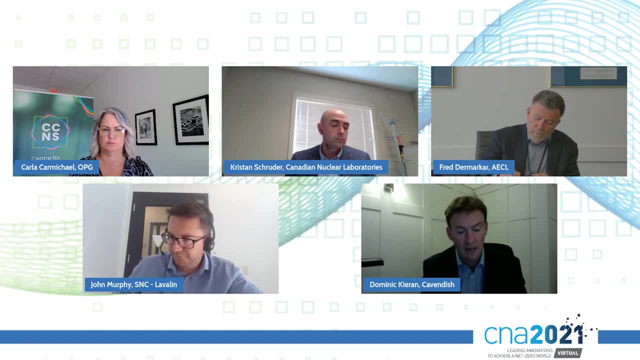 see quite a lot of parallels between uh, between the uk and uh and canada. so very quickly, um, let me just give you a couple of examples. so innovative approaches, um, you know these were demonstrated, uh, particularly in the decommissioning of magnox reactors in the uk. so the the value proportionate. 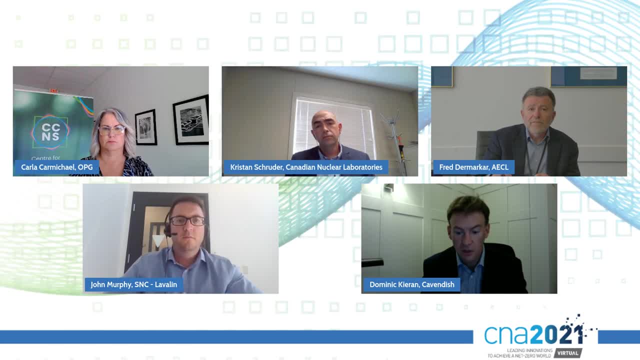 safety cases there, bought huge savings in in time and cost uh at cellarfield some very high hazard decommissioning by. by putting teams together to think differently, um, to think about processes, different approaches, there were huge savings in in sort of uh in in the budget and indeed the 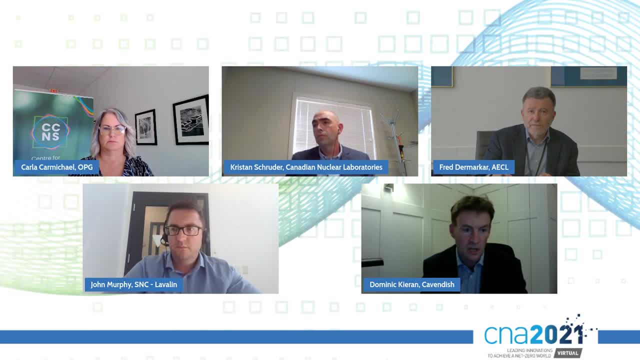 timeline on these really high hazard decommissioning projects. this was supported by technology, absolutely, absolutely. i think, first and foremost it was overall approach. so finally, last comment, i think when i uh, when i look at some of the decommissioning challenges, or maybe opportunities, if i can put it, 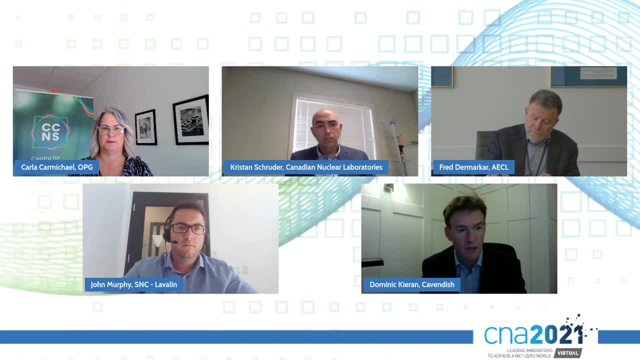 in canada. i see massive value in collaborating to share ideas and, and just to be really clear, by collaborating it's you know, if i think about a uk perspective, i think we have a lot to share, but actually this is about reciprocity. we need to learn as well and bring a lot of. 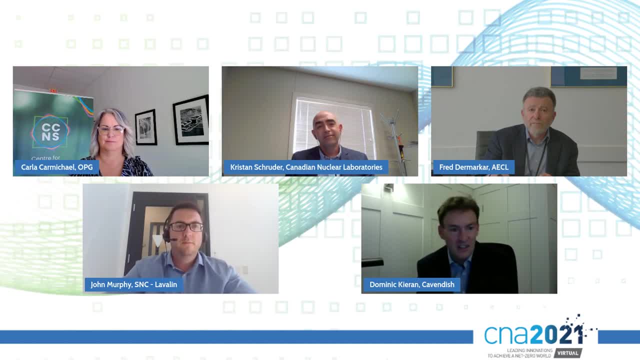 the experiences from canada back into the uk as well, uh, so i think i'll just play a little bit close there and say i think collaboration for me is uh is an exciting opportunity in this area. so, thanks that, that's great, dominic. uh, thanks very much. and and this idea of uh countries learning. 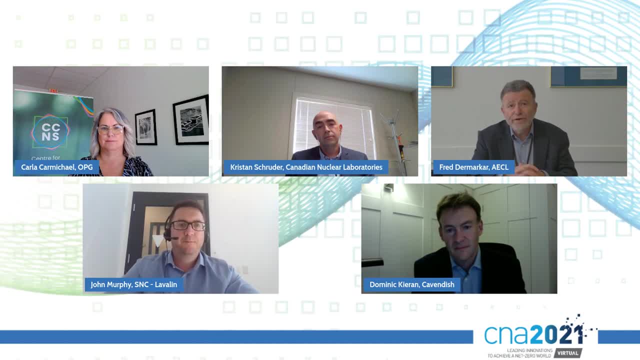 from each other. i think is is central to what we've been doing in nuclear and it has made nuclear better, so it's a great message that we should be doing exactly the same in decommissioning next. uh and last and certainly not least, we have john murphy. uh, john is the vice president. 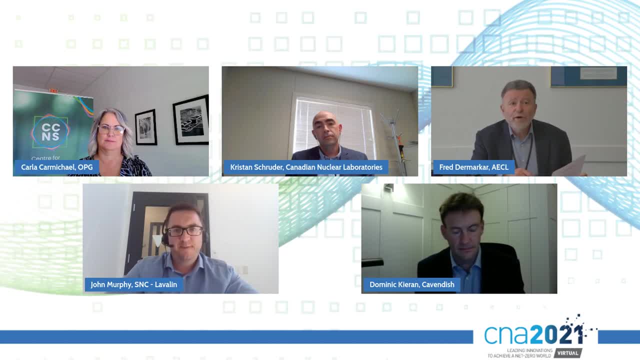 of radioactive waste at snc lavalier. over to you, john. thank you, fred um. i'd also like to thank uh, the cna, for inviting me to participate today and i think i'll start by saying that, in general, decommissioning has its challenges, but, and especially when we overlay the complexity, 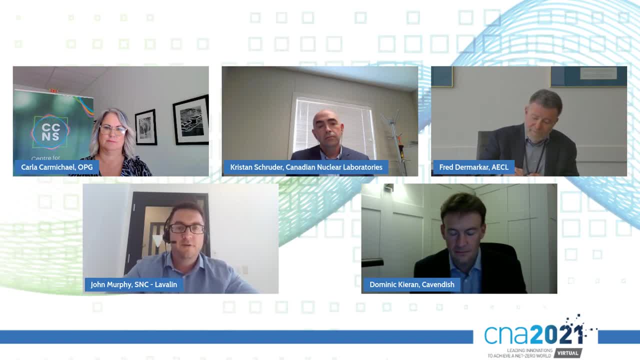 of working in a radiological environment, the challenges we face can be quite unique and, for a number of reasons, when compared to other phases of work, we typically have more unknowns to contend with. in decommissioning, essentially, we're not starting with a blank canvas and we inherit a facility or an asset and, unfortunately, 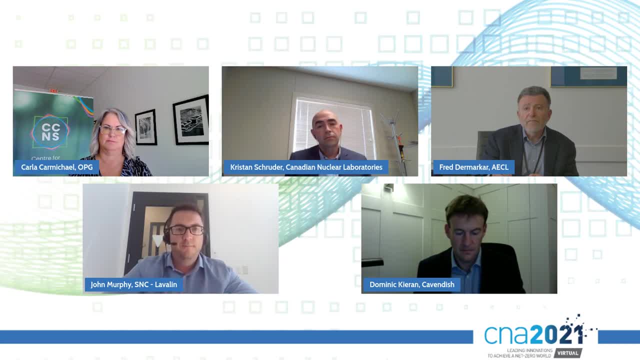 what we sometimes find is that the the actual condition of the asset can be very different to the perceived condition or the recorded condition, and that's something which has tripped us up on more than one occasion in my experience. so, as an example, inaccuracies in plant config data. 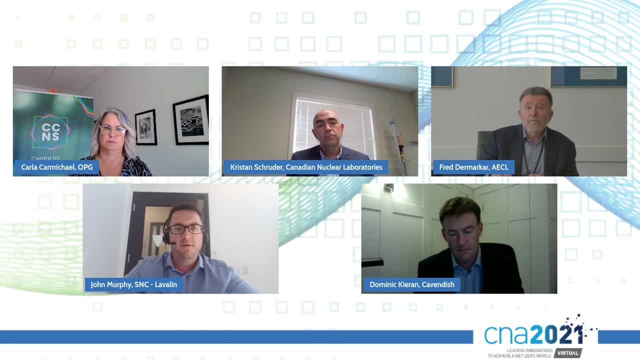 emissions to drawing, updates or installation and minor services that haven't been captured, and these are error traps which we come across in d commissioning that can ultimately lead to rework and therefore increased costs and schedule extensions, which which clearly aren't the objective when we start a project. we have seen some 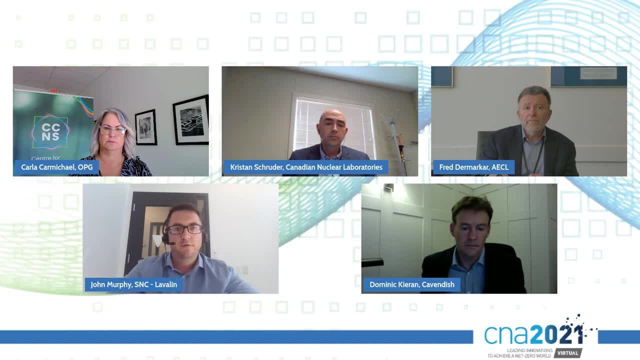 innovations which seek to improve some of those on some of those challenges, and the one that springs to mind is kind of the digital scanning capabilities. that's a prime example of something that's been introduced recently, in the last couple of years, and it's certainly an enhancing the accuracy of our information and removing some of those knowledge gaps and 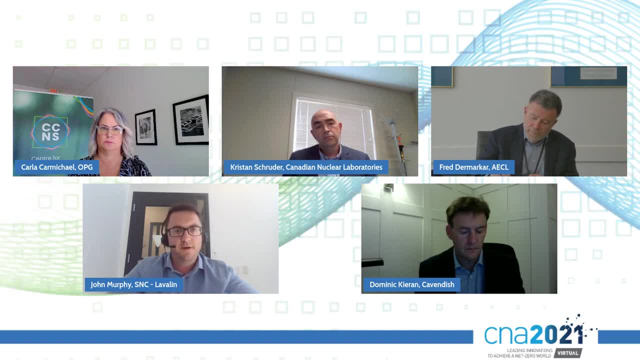 reducing our rework. Therefore, I'd suggest that investment at the front end of our projects to scan, to characterise and to truly understand the environment is a good investment to make, and the savings that we realise from doing that significantly outweigh the costs. 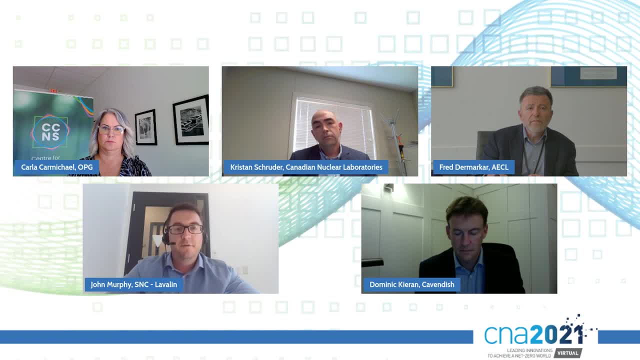 I would probably go as far as to say there should be some consideration given to making that a mandatory element at the front end of every schedule. From my experience, innovation doesn't only come in the form of products and technology, and Dominic just mentioned something very similar. 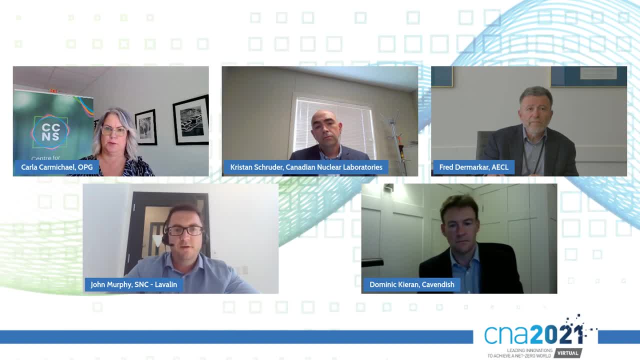 Perhaps of more value from my perspective is innovation in our approach and investment in our people. It's incumbent upon us, as leaders in the industry, to create an environment and a stage which supports the transition of our people from an operations mindset to a decommissioning mindset. 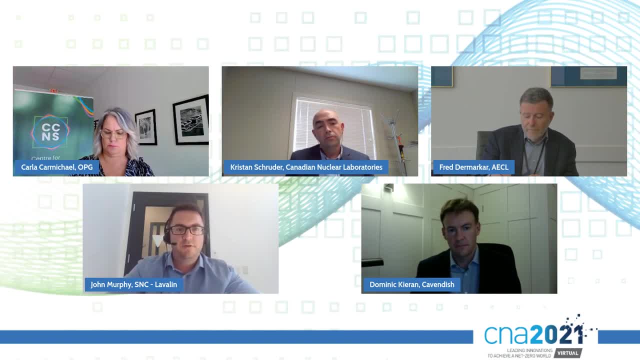 and I guess that it drives the question: what does that really mean? And for me, it means becoming more comfortable with unknowns and the application of a LARP, as Dominic touched on. also, It means becoming comfortable with changing work faces on a more regular basis and providing processes and 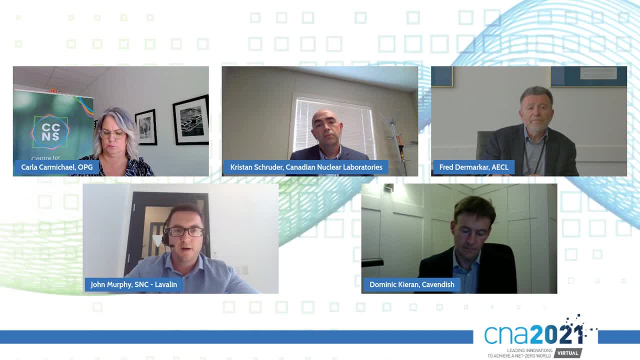 procedures which recognise this and give our people the bandwidth to take appropriate action. It means change to the way that we think. Essentially, we're looking to safely and efficiently dismantle our plants and in some regards, therefore, I'd suggest the thinking we apply to this phase should differ from a new build programme, for example, 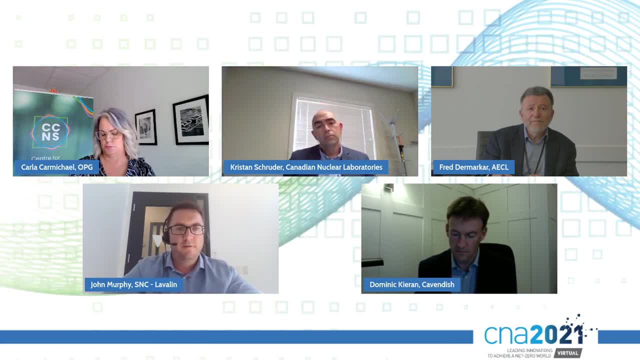 And I guess just on a personal level, having recently arrived in Canada with my family, I've had the unfortunately had to spend an enormous amount of time building IKEA furniture in the past few months and I'm pretty sure my approach to dismantling those items in future 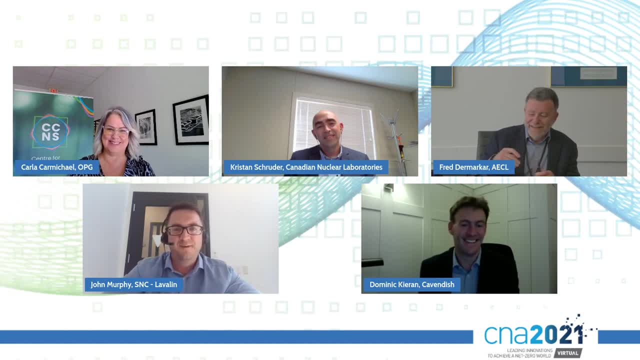 years will differ from the approach I took to constructing them. And not to kind of suggest, of course, that building IKEA wardrobes relates to nuclear, It certainly has. it's an analogy to think about And I'm not suggesting that we take that approach to our facilities. You. 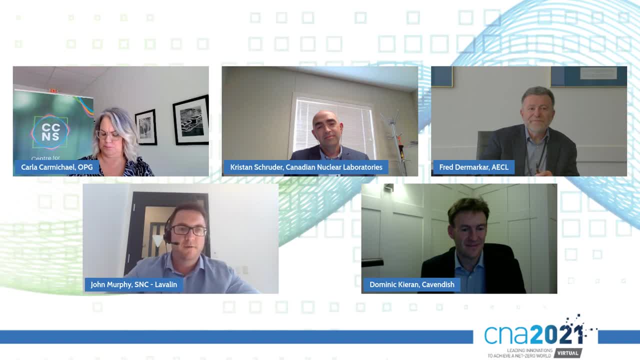 know, conventional and radiological safety has to remain our primary focus. We do have the advantage, however, of taking OPEX from other geographies who are further ahead or further into their decommissioning programme than we may be here. And one key: 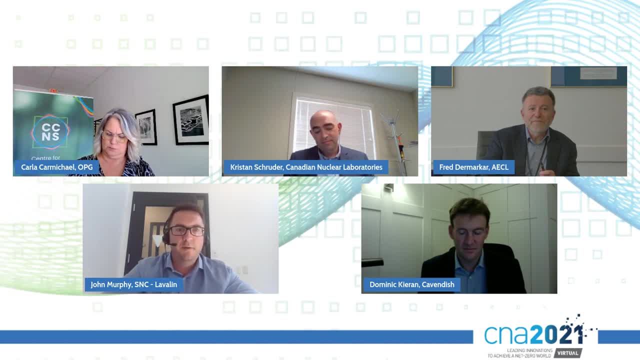 learning that I did take is that seeking to understand every variable before we commence isn't the right answer, Nor, for that matter, is proceeding with an unpalatable level of risk. We need to find the right balance and accept that through doing, we'll adopt a lead and learn. 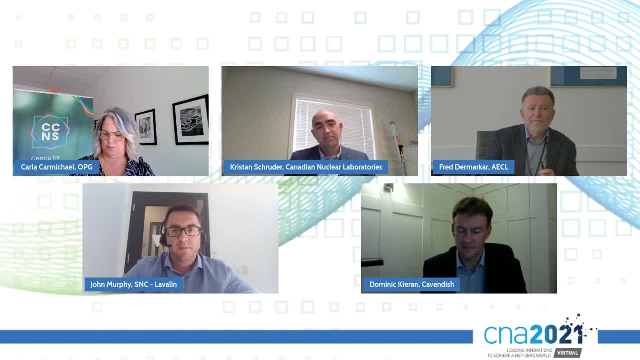 approach And I think we have to accept as an industry that we're going to make mistakes but we will benefit from those mistakes and from that learning in the fullness of time. In the UK we certainly got that balance wrong at times and this led to some significant cost. 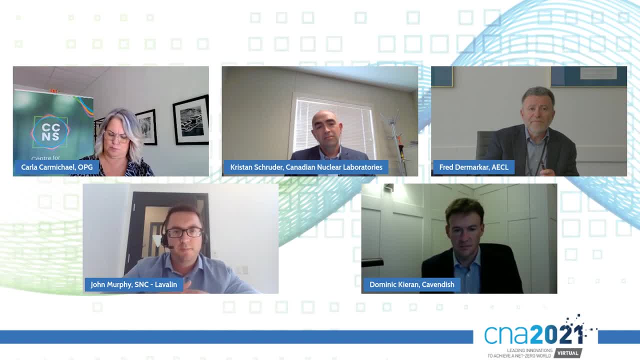 and schedule overruns, And we shouldn't be ashamed to take that OPEX and use it to our advantage in Canada. I'd also like to touch on the narrative associated with decommissioning. We often refer to the need to speak more positively about nuclear and its benefits to the general public. to 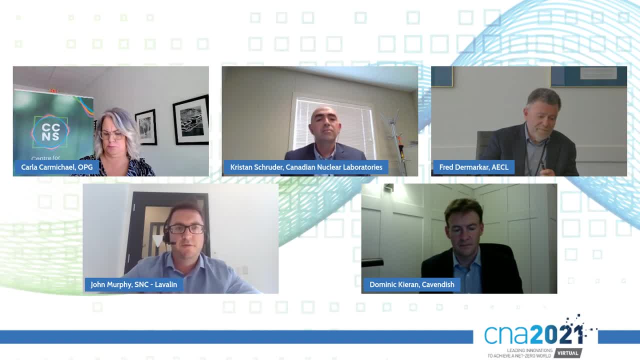 enhance their understanding of our industry and to remove some of the misconceptions that exist. I think the same can be said for decommissioning, not only externally but also within our industry. Whilst, by its very nature, decommissioning falls towards the back end of the nuclear life cycle. I feel we could better our 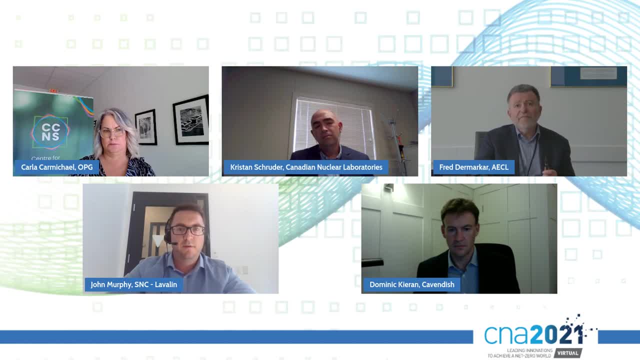 articulate the importance and benefits that effective decommissioning can bring. To achieve this, we need to invest time in getting everyone a message with a clear mission and purpose for decommissioning. This is something which drove a step change in delivery performance on a program. 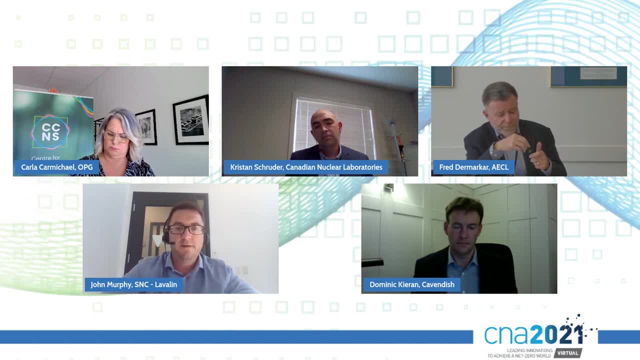 I previously worked on, and the impact of the risk of not doing this and having working groups with different views and agendas will impact far greater than any other factor. The final thing from me is that clearly we carry a responsibility to clean up our legacy facilities, but in doing so, we have a fantastic opportunity to demonstrate to our stakeholder groups. 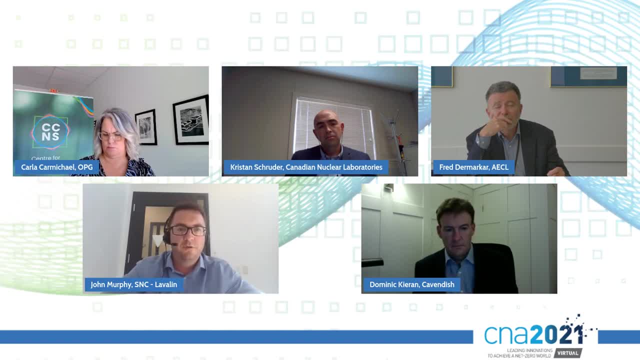 that we know how to manage this phase of work and we shouldn't underestimate the importance that is driving confidence into new investments and ensuring new nuclear is a key component of our future energy mix and our aspiration for a net zero future. Thanks, Fred, Thanks very much, John. I must say some of the comments that you made very much resonated with. 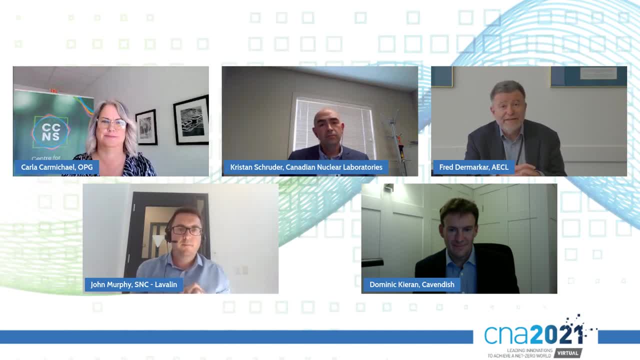 me. My background is in nuclear operations, not in decommissioning, and we're used to having a much higher level of certainty than the decommissioning group, where we're dealing with wastes that were generated 70 years ago and where the records are not quite as good as the 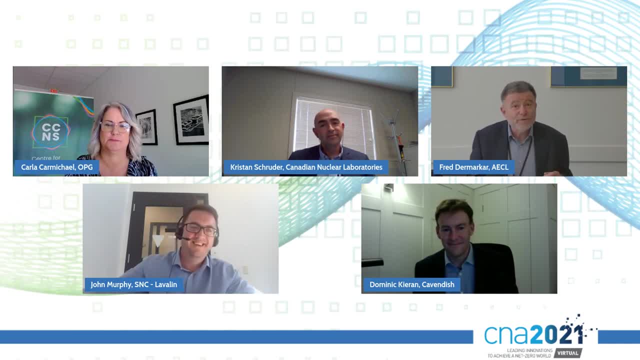 ones that we kept at our nuclear plants, and it does pose some unique challenges. So I thank you all for those Those great comments. to start us off, What I'd like to do is I have a few questions here, and I'm seeing that we're already getting some good questions from the audience, So we'll start off. 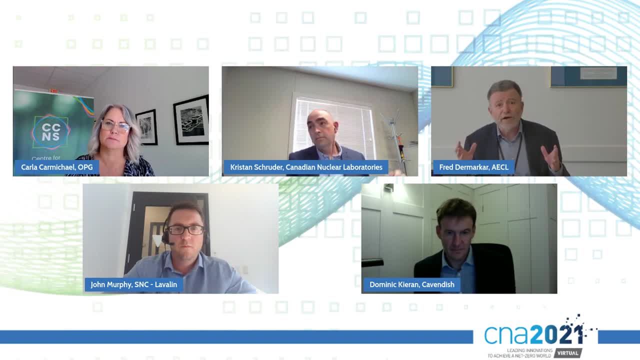 Dominic touched on this, but I'd like to give everyone an opportunity to elaborate on: what experience do your respective organizations have in bringing into the Canadian market approaches that can make things safer, faster and more cost effective and lower cost, And maybe what we'll do- Carla will start with you. 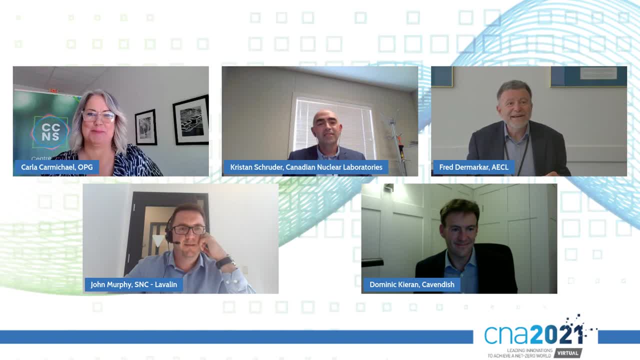 You're on mute, Carla. I knew that was going to happen. Yeah, so we are in the Canadian market, but I think what we bring is we have 50 years of already safe, clean, reliable, strong performance in this industry, so we provide that. I think that that. 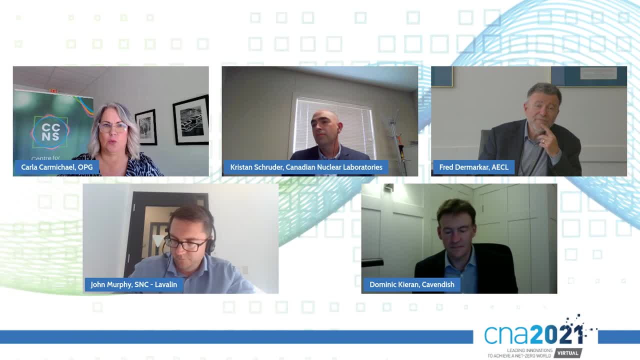 provides the stable table stakes to do sort of the work we need to move forward and apply innovation and new ways of thinking. We've proven this through strong operations. at Pickering Darlington I would say Bruce Power, I know that's not OPG but of course a significant 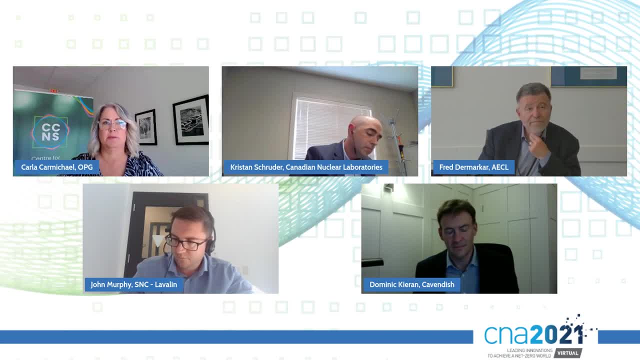 part of the industry, But we've also proven it by being able to execute large projects very well, And so the Darlington Refurbishment Project is one of them, as well as Bruce Powers MCR project. Those are progressing safely, on time on budget, And I think that that 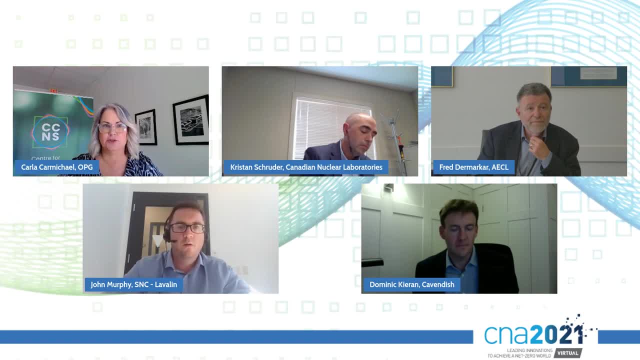 provides us with that social license to continue doing these big projects like we're going to have to do with decommissioning or with pickering and hopefully SMRs as well. We do a lot of benchmarking, lessons learned reviews, but we also 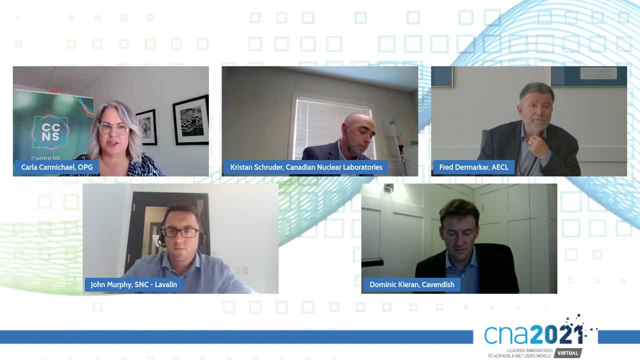 don't feel that OPG can do this on our own. Again, this is what I've said at the beginning: we are not decommissioning experts and we need everybody to work together and help us do this, But we also engage. 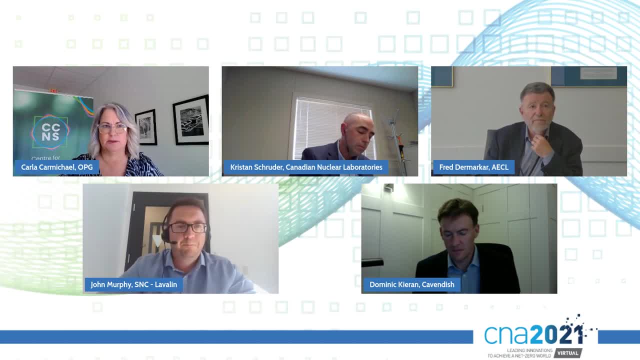 and get input from our communities. That's really important- The communities that host us that may host future activities, but also our First Nations communities. So we have to lay that framework. We're strong in the Canadian industry, in the market, but we also have to keep building on. 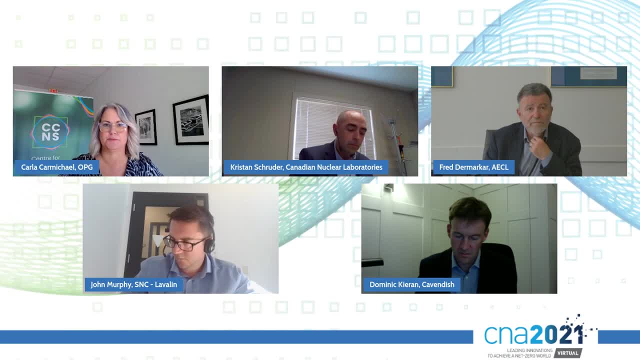 that framework, I think, to do what we need to do. Okay, Thank you very much for that, Carla Kristen. what are your thoughts here? Yeah, thanks, Fred, And you know, I think what I would point to for this question would be the: 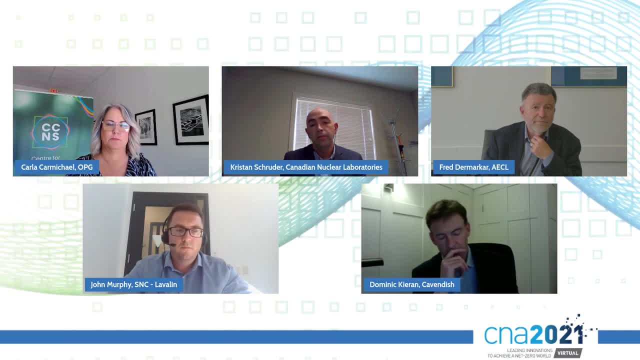 GoCo model that Government Canada brought in through ACL for CNL and how that has helped us move forward with our decommissioning and waste management activities here and really start to accelerate stuff. And you know what the GoCo brought in: government-owned company operated. 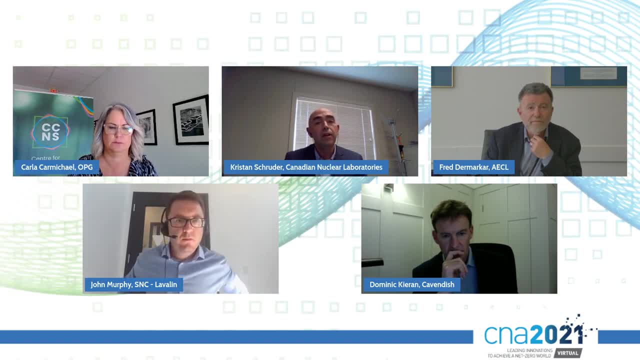 was, you know, a lot of experienced leaders and staff that have been doing this type of remediation work with some of the similar challenges at sites in the US and the UK. So bringing in that sort of expertise and knowledge just helps build the confidence of the staff that 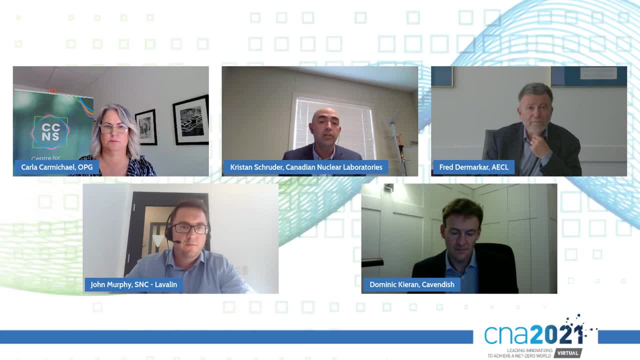 are doing that because we had been doing decommissioning waste management activities prior to this GoCo coming in, but it was at a smaller scale, So bringing in those international experts really helped us up our game and increase the amount of staff that we had working on our 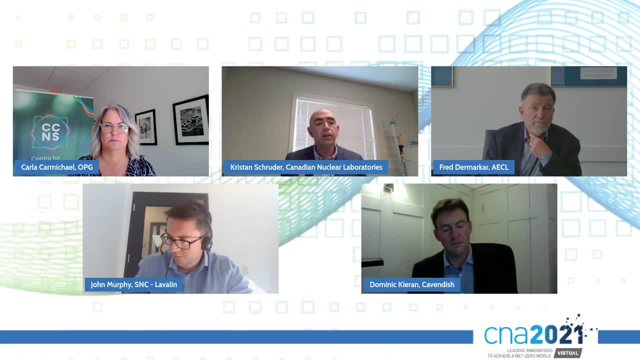 projects And help us really understand how we needed to be set up as teams, with an integrated team, so that we were getting that learning from the various parties, because, as John pointed out, and Dominic, there is a lot of unknowns that need to be managed. So there, you really need to build. 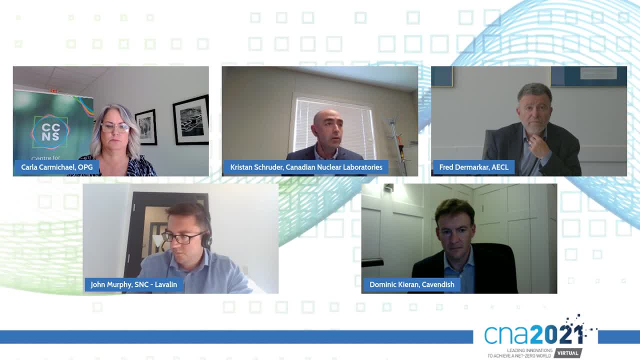 that integrated team in order to do that. I think, the other thing that I would point to- and Carla mentioned all of this benchmarking- you know, so we do a lot of benchmarking here at CNL And that is, you know, with organizations such as SNC and 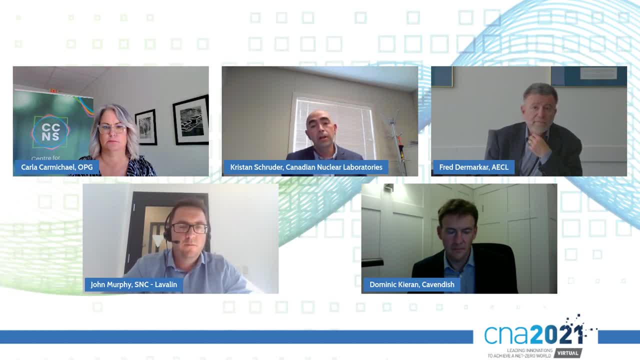 Cavendish, you know the UK and Europe has been doing a lot of decommissioning and so has the US. So every opportunity that we have to benchmark against other projects, similar projects, the community is very open to benchmark. It's one of the things I've noticed, that 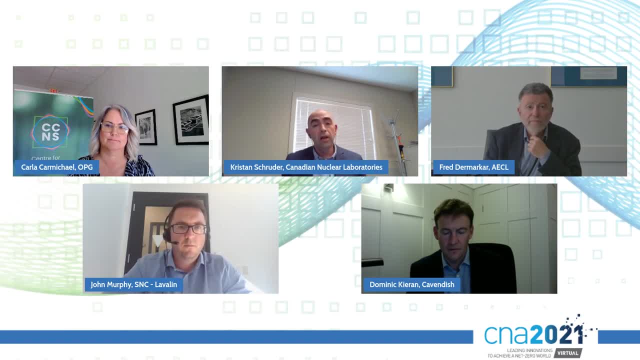 you know, a lot of people in sight are open to having visitors come in and learn a little bit and sharing right, collaborative and, just as Dominic pointed out, right learning from each other. So that's what I would say, you know. 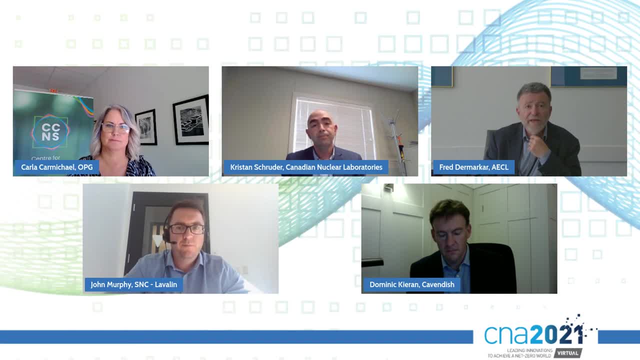 included as part of my remarks to that question. Okay, very good. Thank you for that, Kristen. We'll go to John next and then get Dominic to offer us his last thoughts on this, because he introduced the subject in the first place. 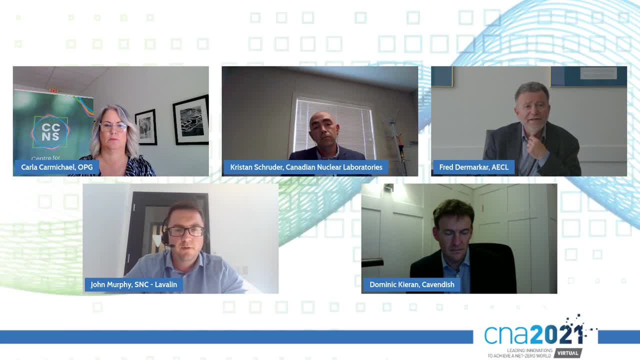 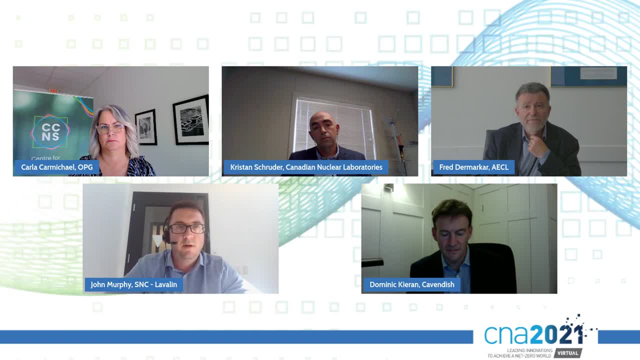 collaboration is a really important one, And one of the key learnings that I bring to Canada from the UK is that where we had the most success is where we set up alliances. that involves a number of organisations and the client, So kind of the site licence holder was one of those. 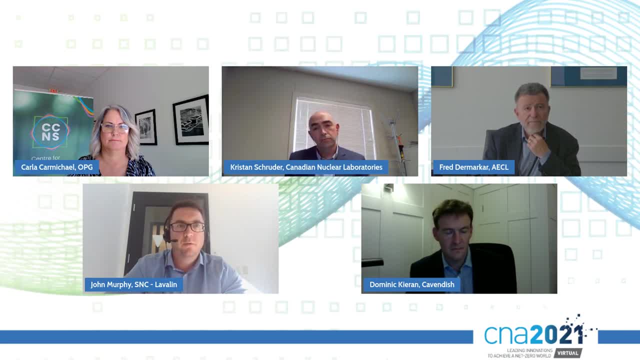 partners in the arrangements, And what that allowed us to do was to build a level of transparency and trust and move the relationship away from a transactional one and to a more were far more. as kate christian just mentioned, we were operating as an integrated team and that 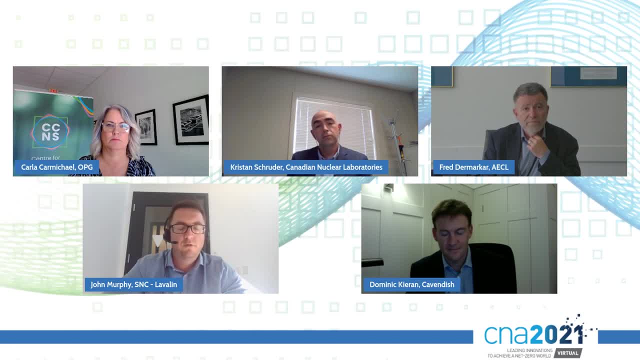 allowed us to get things done far quicker. um took away many of the barriers and we made you know much greater progress by adopting that approach. great, that's. that's great to know. thank you for that, john, and, and now over to you, dominic. yeah, fred, fred, thank you. so i don't want to repeat. 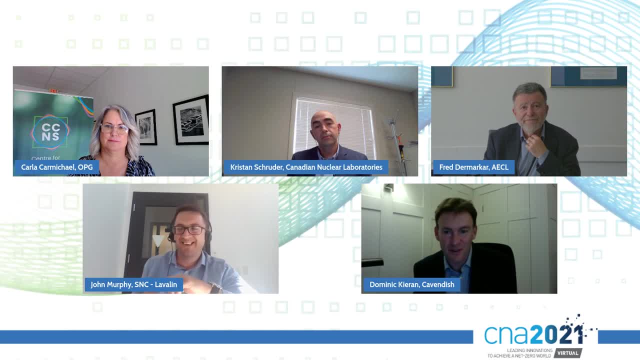 because actually, um, um sort of three colleagues have stolen most my answers by uh like before me, but but maybe just one. um. one sort of final perspective is, i think it's back on this idea of collaboration and, i think, on the mega projects that we all get involved in, um, i think things like: 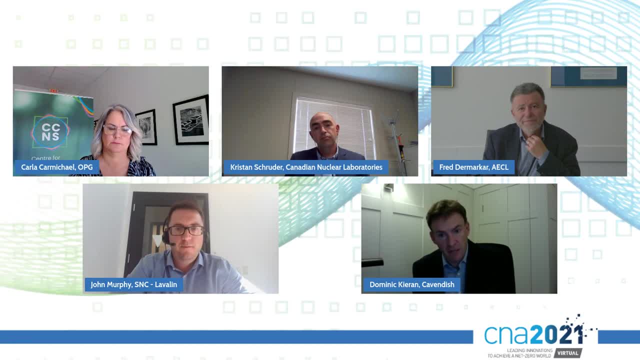 a risk-based decision-making approach to decommissioning is key, particularly, as i said, in the regulatory environments that we have now. that's kind of quite an academic concept, but actually i think it's most powerful when you've got the sort of practical battle scars behind you, and that's actually where sharing and learning 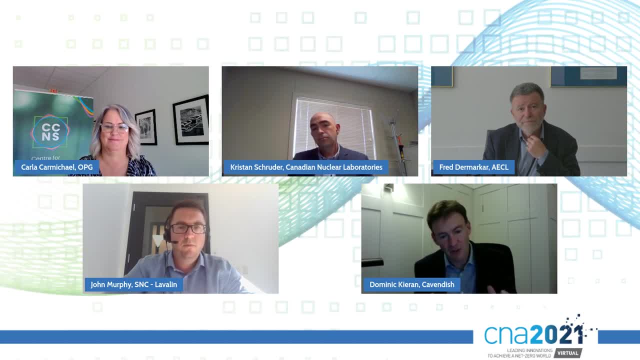 really, really help and if we're looking at these projects, that there's a lot of integration needs to be done. you do need to bring in technologies, you need to bring in, uh, innovation, um, but, but an interesting- this is just my final thought- an interesting facet of doing this correctly. 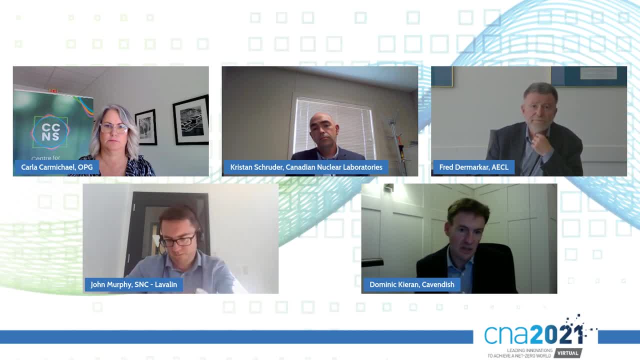 where you've got some experiences. it opens the door to do things like bring smes into the fold, and so one of the things we're really keen on is actually leaving a legacy and leaving a footprint in the areas that we're we've been operating and one of the ways you can 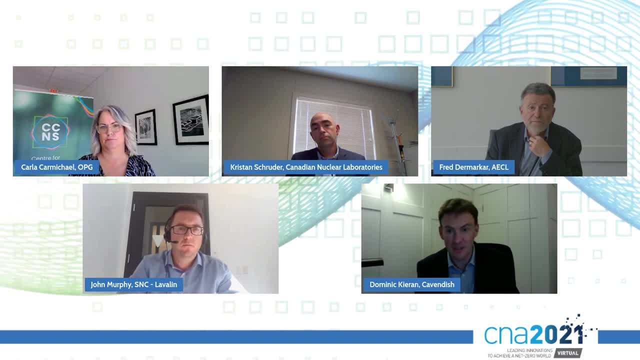 do that is bringing smes in, helping them be successful in these sort of mega projects. i think that is sort of enabled by this sort of risk-based approach, which in itself is enabled by kind of having been there, done it before, made a few mistakes and, uh, they got a few battle scars. 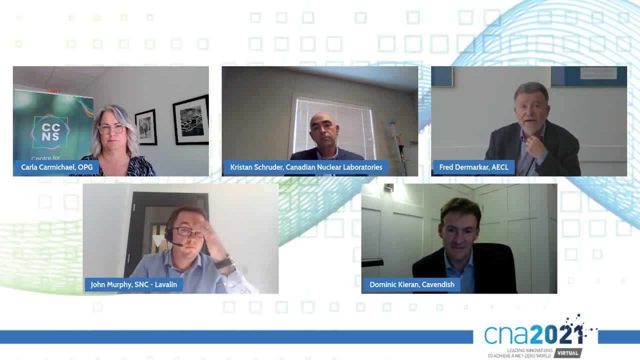 right, and by smes i think that you mean small and medium-sized enterprises, as opposed to subject matter experts. thank you very much. absolutely, i do, fred. i should have clarified that. i appreciate that. no, that that that's great. uh uh, kristen, there i'm gonna ask you a very quick question because i think it's a very quick answer. 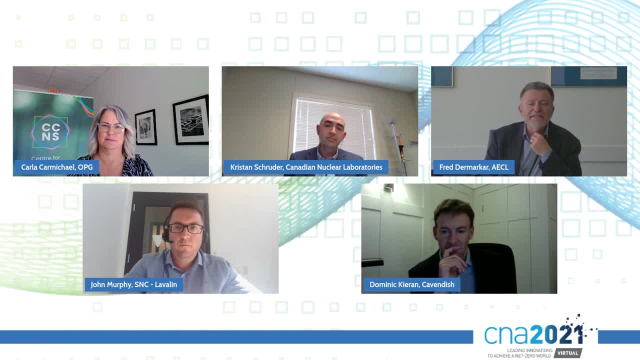 from the to to an audience question: how many of the 1600 or so staff, uh, at cnl are actually there's? let me correct that there's about 3 500 staff at cnl. how many are from outside canada is what the audience is asking. 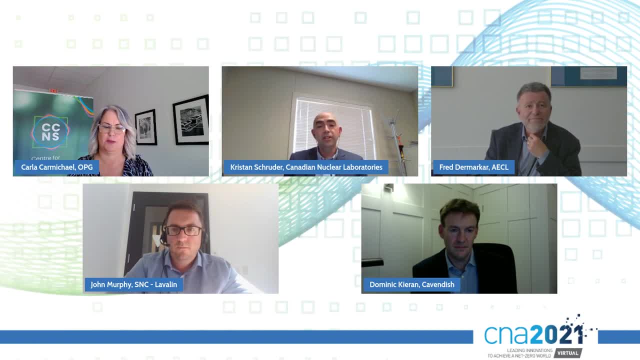 uh, you know, it's only about a couple percent and that's largely in leadership and supervisory roles that we have from outside of canada supporting our decommissioning program. okay, perfect, and and and i'll pose this question and if you want to put up your hand to answer it, uh, i don't. 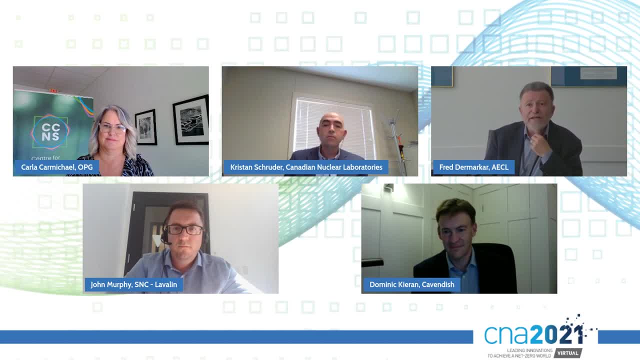 think we need to go around to all four. it's another audience question and uh, and the question is uh, do the challenges of a decommissioning project require a new talent pool or supply chain, or can you leverage the existing employees, union workers and suppliers that are in the market today? 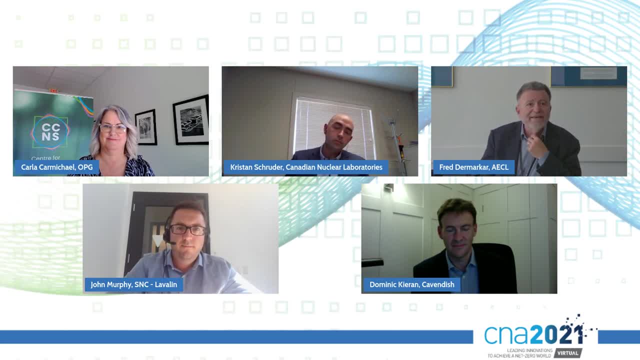 so, whoever wants to answer, just put your hand up and uh, yeah, we'll go to. well, it looks like all of you want to answer, so we'll. we'll start with kristen and uh, and then we'll go around the loop. sure, i'll be quick, um, so you can absolutely. 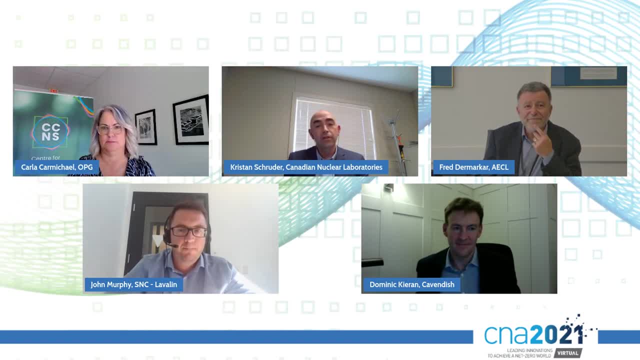 utilize uh leverage existing employees, union workers and suppliers. uh, fred, you know so and we've demonstrated that at cnl um we are. our decommissioning workforce is is largely coming from either our operating uh, operating uh workforce. they're coming from the science and technology workforce. we have hired in new people uh, but you can absolutely leverage existing 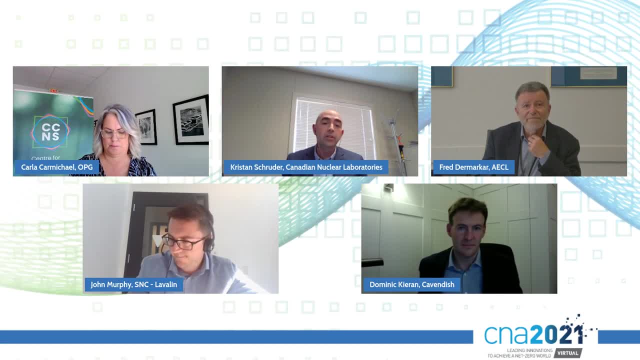 employees and you want to leverage existing employees because they've got the tribal knowledge and the plant knowledge. that is very important to move the decommissioning program forward. so i'll i'll leave it there because everyone wants to see it. anybody want to add to that? 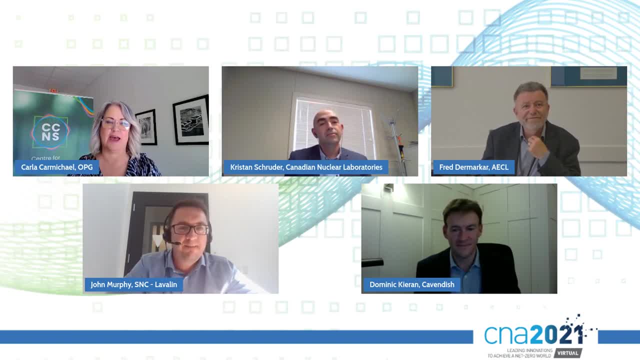 carla, yeah, i was just going to add that this is interesting question because innovation, um in collaboration, can be done on many things and and in fact, the the four of us are actually collaborating on this very question. interestingly, um and um, we were, we are working. 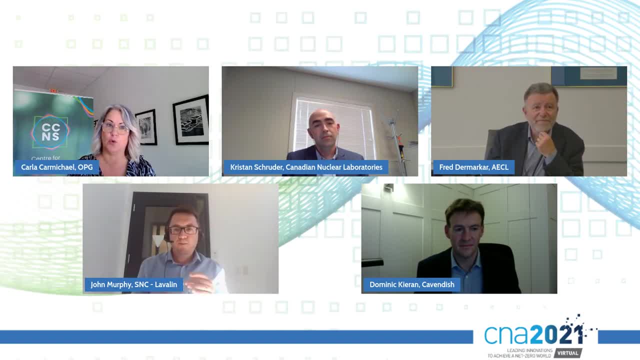 together, particularly since the fact that we are a small organization. we are collaborating with them. we are working together, specifically since the fact that we are a small organization, we are working. CNL, OPG to understand sort of the roadmap for the next few decades and understand the demand. 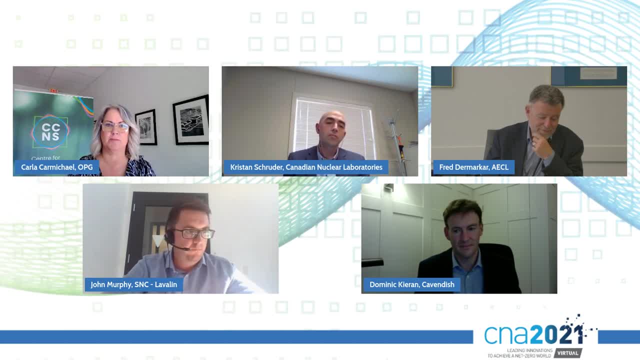 supply what kind of skill sets we're going to need. over time We're reusing, you know, Cavendish's expertise in doing these big projects to understand, kind of really what kind of skill sets we need. And then we're looking at, you know, how can we develop and retain the skilled workforce we have. 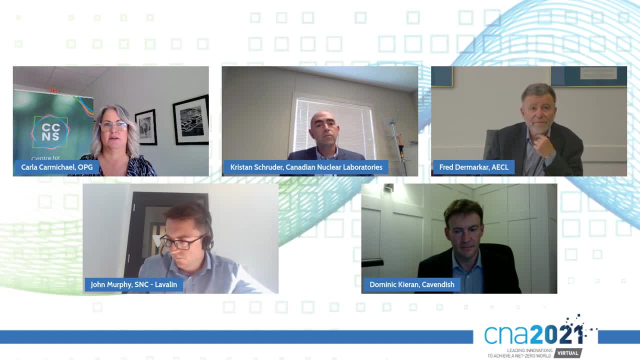 in the Canadian market now, And if reskilling is needed that's fine, But many, many times that's not necessarily necessary, And then progress them over that 20,, 25 years. We want to show the nuclear community and the supply chain that there's a lot of work ahead of us and good work. 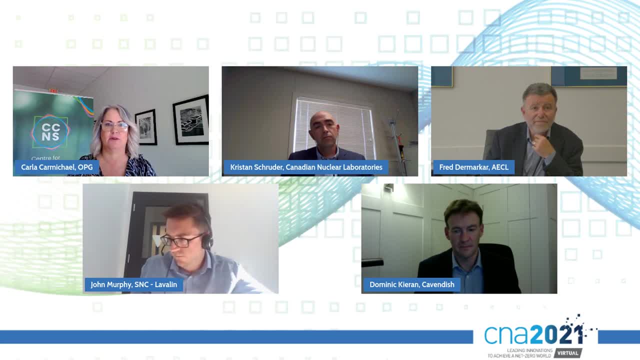 And that by working together we can figure out this challenge right, Having the right people at the right time, the right work and creating that industry for workers and supply chain. So it's an interesting question because all of us- actually the four of us- are working on. 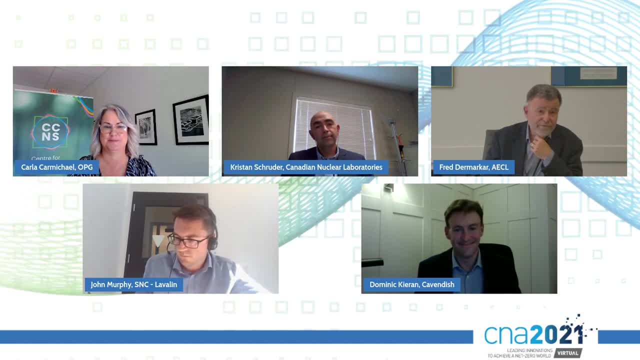 this particular topic together. Very good, Very good. Thank you, Carla. Anybody want to add to that? or are we good? It looks like it looks like we're good. So another question is: you know the whole theme here is. 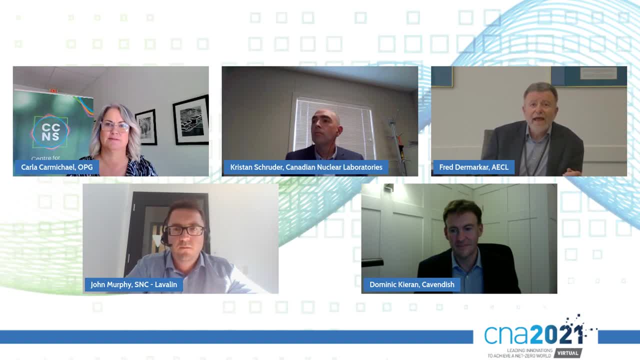 around innovation and in decommissioning, And at the CEO discussion that we just heard, it was clear. Romina Velshi indicated that the regulator very much wants to enable. They don't want to be a disabler to regulation But, as Dominic noted in his comments, we need to prove. 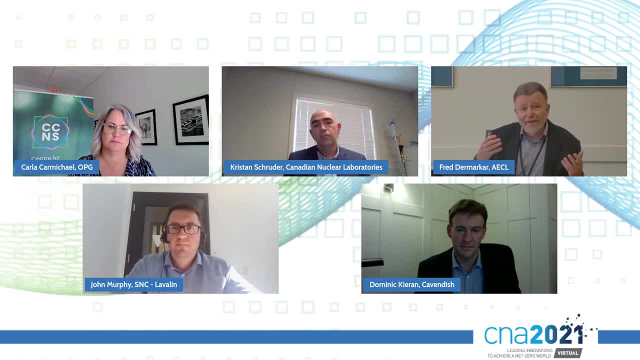 that the innovative approach is safe, And there are challenges there because it's something new, it's different, And so can you share ideas? Yes, I can share ideas regarding how do you introduce innovation, demonstrate that things are safe, but do it in a manner where we can actually very efficiently get to where we need to get to. 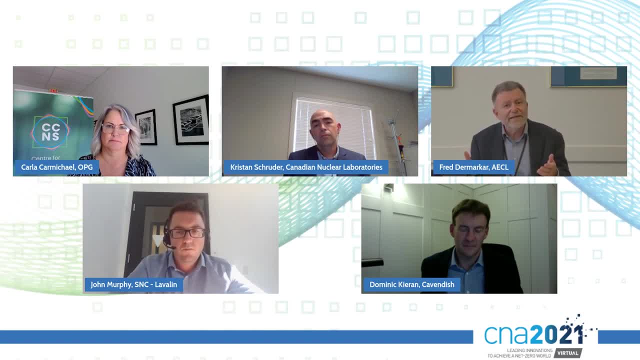 because demonstrating that something is safe is a lot easier said than done a lot of the time. So maybe, John, we'll start with you, And do you have any thoughts on how we introduce innovation in such a way that it will clear regulatory requirements in a very effective? 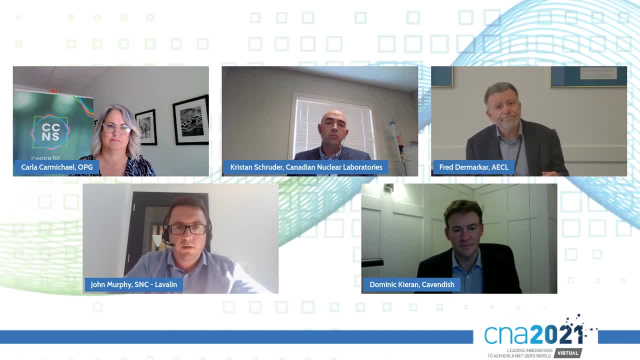 way I can take a go at that, Fred, from our experience, And I think what I would say to that question is is that ultimately, you know, when we're dealing with regulator, we need to recognise that ultimately they're there to help And by recognising that and taking perhaps a stage of the 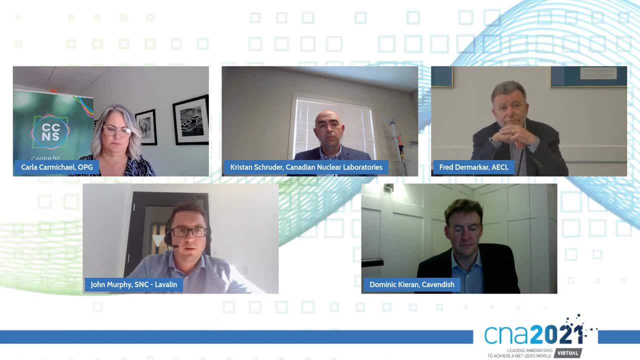 approach and really bounding our scope as we, as we look to try and introduce new technologies And as we move forward, make sure that we gather data to remove some of the pessimisms And, if that means, for example, taking some lab scale testing before stepping into inactive 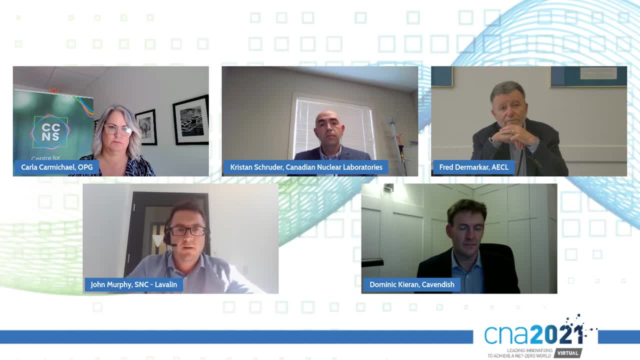 testing before active testing and then field deployment. ultimately, I think these are the kind of the sequential steps that we need to take just to make sure that we gain confidence as we go through that process. Very good, Thank you, John, Dominic. your thoughts on this? 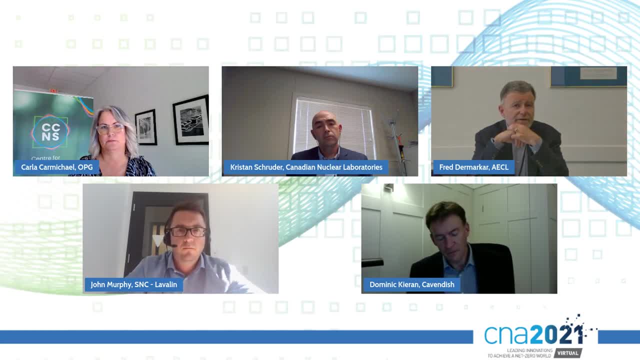 Yeah, sure, No, I think that's a great question, So so I think my answer is quite simple. It's one is it's about regulatory engagement, And so I think first of all is respect that we have different roles to play, But actually very, very early regulatory. 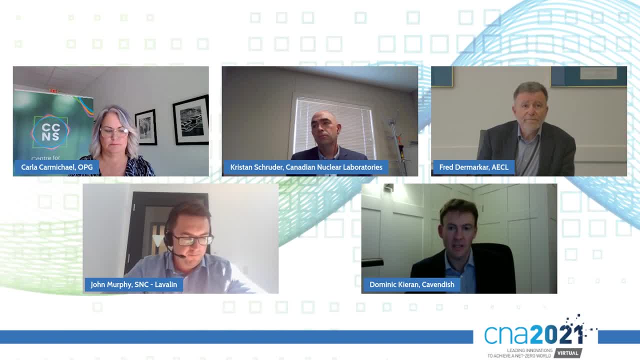 engagement is a one team approach, I think is key because at the end of the day, nobody wants to do something that's unsafe- Nobody at all. So actually we've all got the same vision here, I think. for me it's about the taking away the sort of blockers of bringing in new 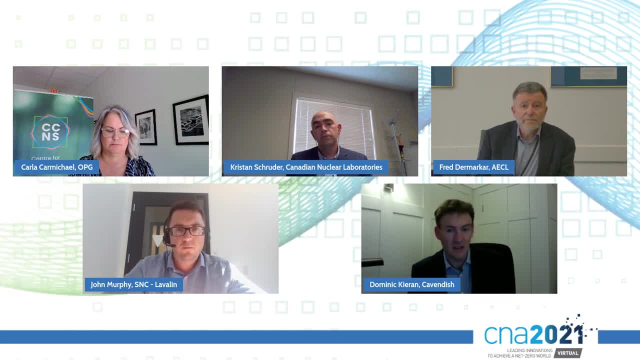 approaches And the way to do that I'll be- I'll be succinct, I think- is simply respect. we've got different roles, but it's early engagement and it's one team Very good. Yeah, no, I. it's a great point, Kristen. 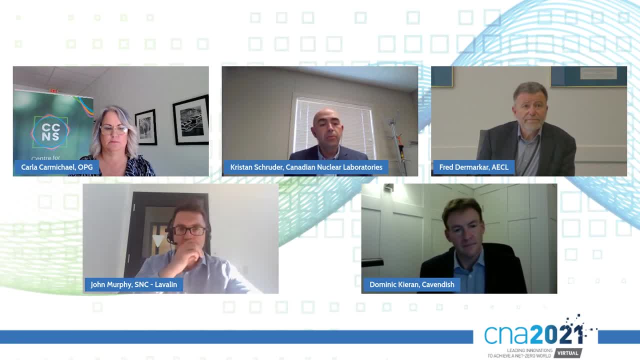 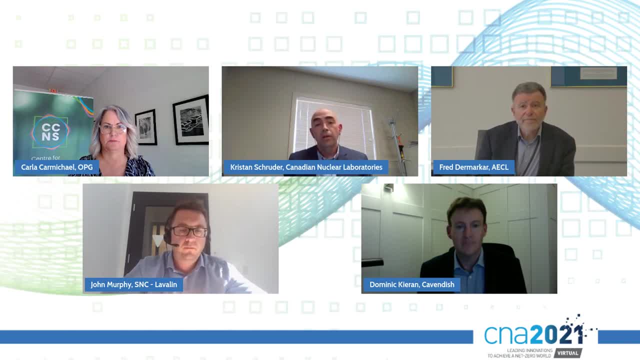 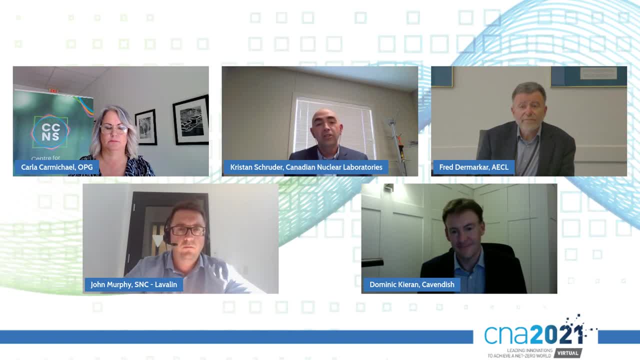 more innovative on your high hazard activities because there's a lot of uncertainty and it could be introducing some risks. So you know, starting that on a low hazard activity so that you can control the work and demonstrate that what you're proposing to do and want to move forward with. 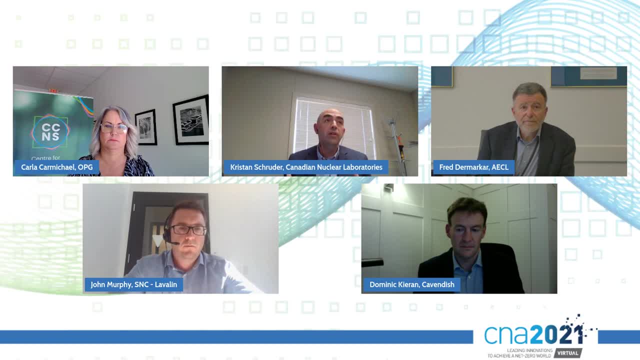 can be safely managed And I think that helps you know. it helps you know for management and ourselves to feel confident. it also helps the regulator as well. So we need to. we need to demonstrate to the regulator that we can do this in a lower hazard environment if we're trying to. 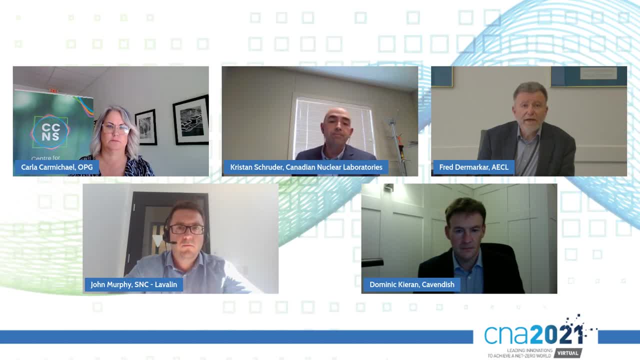 move that forward into a higher hazard environment. So Excellent, Yeah, Well said. And, Karla, anything to add to any of these insights? Sure, I mean we've. we heard President Belshi talk at the World Nuclear Association symposium. We heard her talk today about. 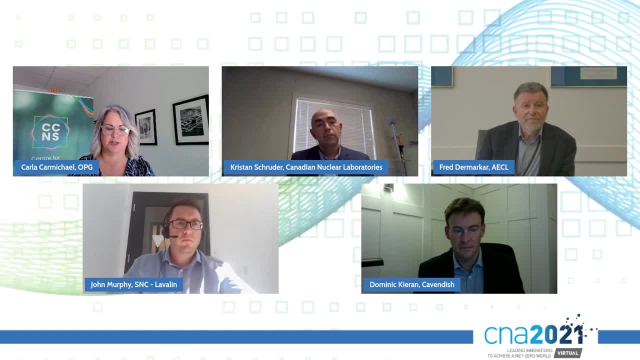 and I love the phrase. the regulator is there to protect the public from risk, not from progress. Yes, So I think that that is really key to remembering And, like Dominique said, early engagement's key. I mean, they're just like any other entity They don't want to be. 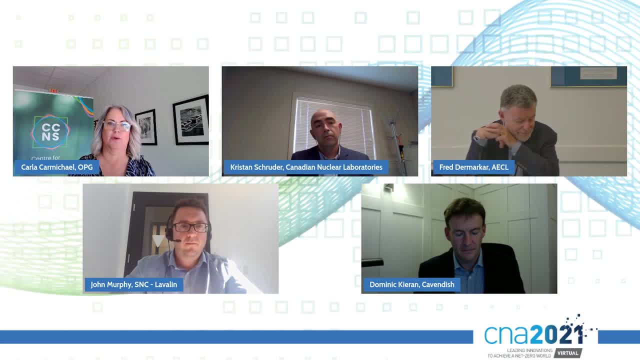 surprised at the end of the day either. They want to. they want to come along the journey with us and help And and and respectfully. obviously we should not shy away from maybe challenging some of the sort of the way things are because, like you said, Fred, you're used to an operating environment. 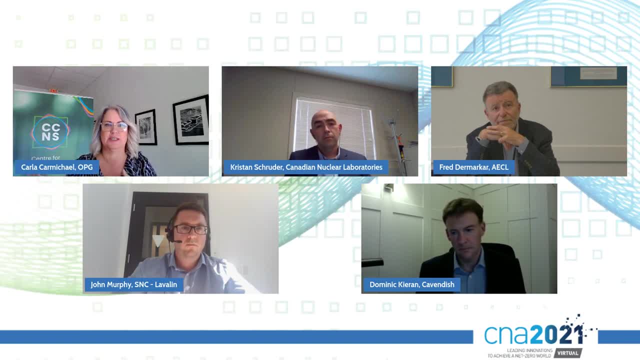 right And and we need to think of: okay, we're going to move to a decommissioning environment. How did they do it at you know? how did they do it at CNL. How did they do it at Cavendish? How did? 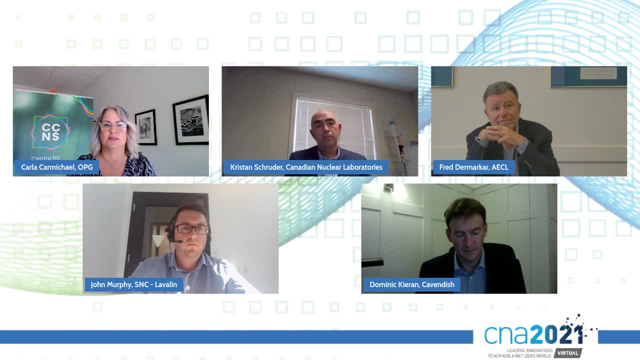 they do it around the world And and bring that lessons learned even with us and and and work with our regulators to, to, to learn those things, And the only way you can do that is to start early and engage them early, And so I totally agree with what Dominique said there as well. So that's. 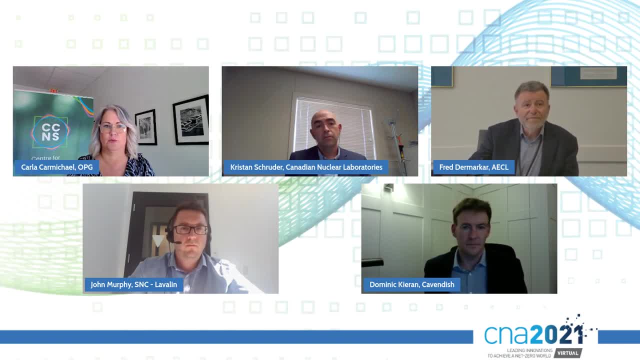 that will be our, our approach as we move forward with planning the decommissioning of Pickering. Okay, Very good, Very good. We we've only got four minutes left, So I I'm going to go to a question that looks ahead And we're in the process of either doing a lot of decommissioning or about 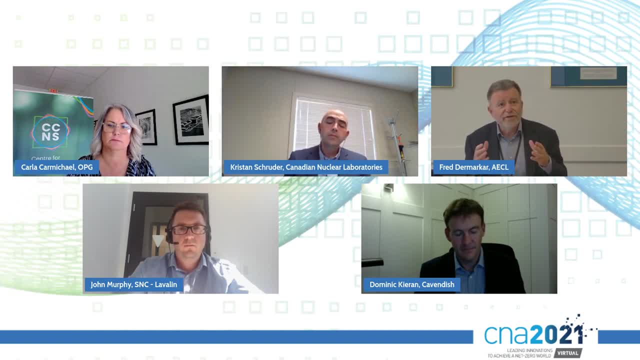 to embark on a lot of decommissioning. So, Carla, you're about to embark on a lot of decommissioning and Kristen's right in the middle of doing a lot of decommissioning. So how can we leverage the experience that we're gaining here? 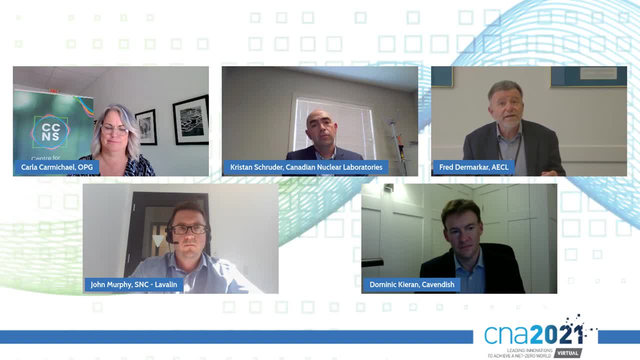 in Canada to compete in international markets so that we can make the most of of of our learning right here. And, and, and maybe I I'll start- I don't think I started with Dominique first on any of these, So 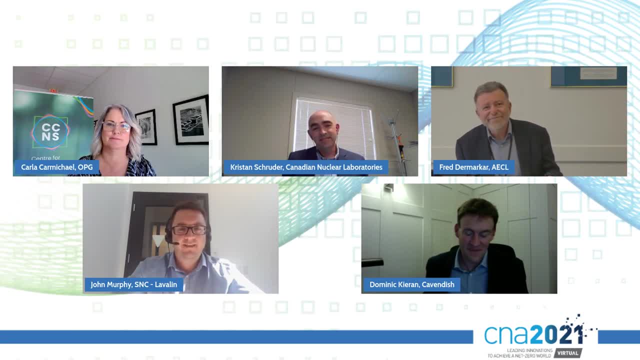 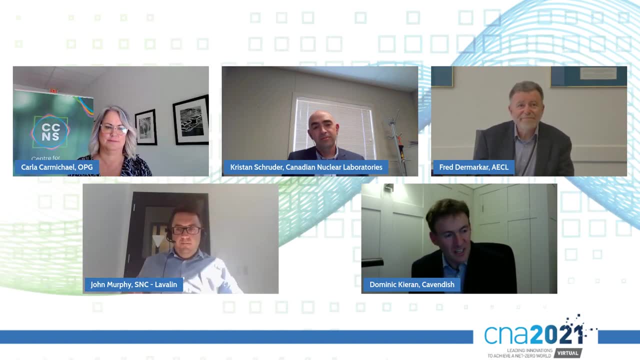 we'll start with you, Dominique, on this one. Yeah, Fred, thank you. So so I mentioned the words of reciprocity earlier, So I think what's very interesting here is there's quite an interesting role of support that we can get from our governments. 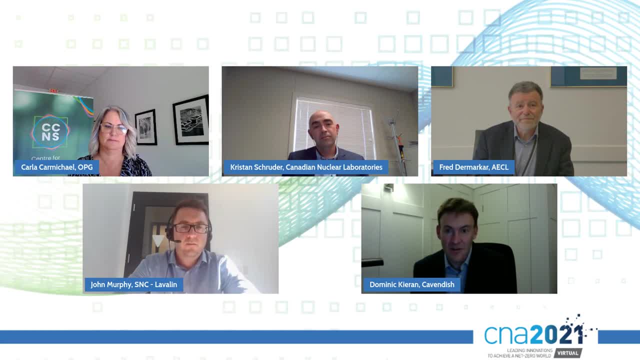 here to enable a lot of this sort of sharing across international borders. And so I think you know I chaired a sort of UK-Canada working group for for nuclear and actually our intention there that this isn't a one way diode. 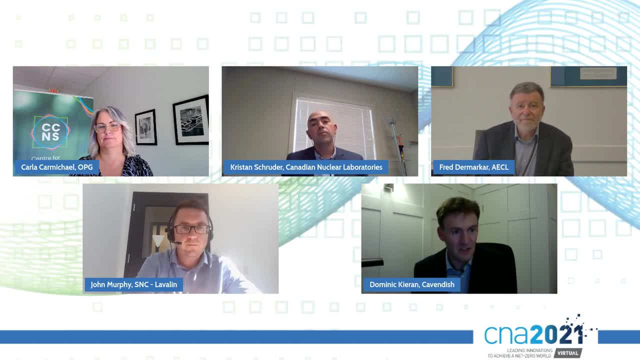 It's actually a show and tell of what have we got on both sides of the Atlantic and and how can we help each other. And what's great is that's being enabled by some of the existing sort of government to government channels And I find that really extremely powerful in just enabling those conversations and getting them off the ground. 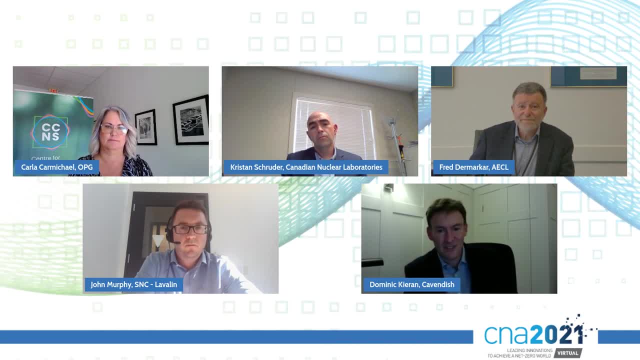 So that's a a sort of a thought to kick off the discussion from me. Fred, Excellent. Thank you, Dominique, We'll go to. we'll go next to uh Carl. Thank you, Dominique. Uh, we'll go to. uh, we'll go next to uh Carl. Uh, we'll go to uh. we'll go next to uh, Carl. Uh, we'll go to uh. we'll go next to uh, Carl. Uh, we'll go next to uh. we'll go next to uh, Carl. 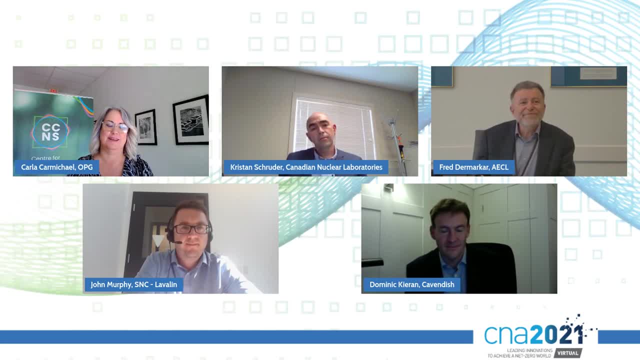 Uh, we'll go to uh, we'll go next to uh, Carl. Uh, yeah, Um, people know my favorite expression is competimates, right? I think you know when we say how do we compete in international markets. 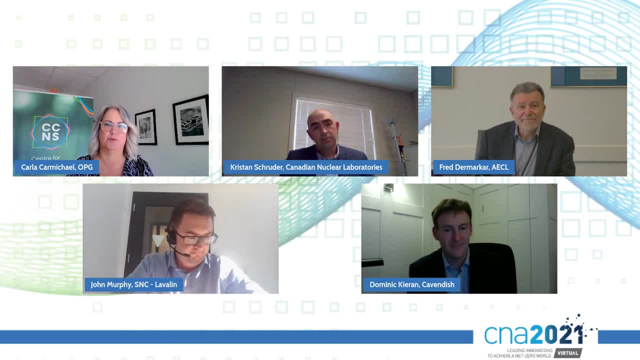 We, we have to actually collaborate in international markets and we all bring different perspectives and and um and expertise, Um and um, and and. Canada has obviously a very strong foundation. We're very good, great reputation internationally. 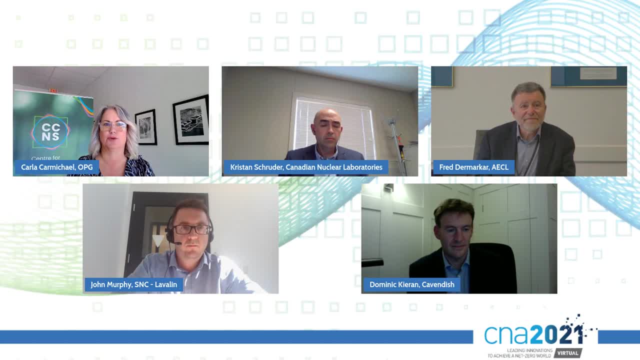 Uh, due to you know our strong operations, our projects, our future SMRs. you know the renaissance of nuclear in Canada. I think that's great, but but we do need to make sure that, uh, we understand that it's it's collaborating internationally as well. 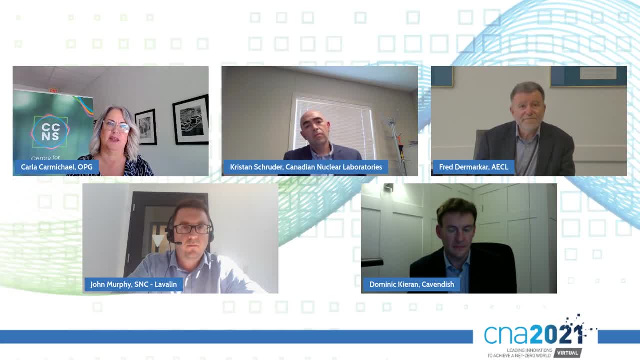 That will make us all successful. Right And um and, and I always say, the pieces together make a better whole. So Very good. Yes, Thanks for that, Carla. Uh, John, And then we'll wrap up with Kristen. 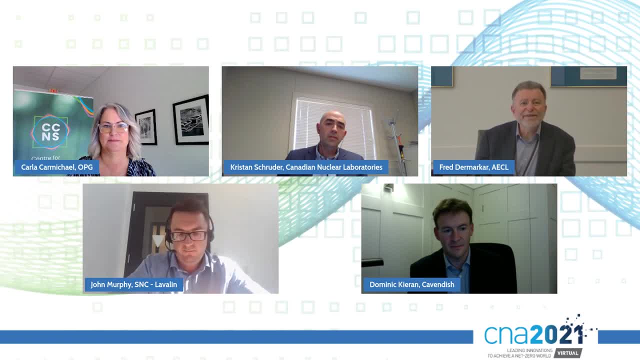 John, Yeah, I think you're on mute. You're okay. Okay, Thank you, So very quickly from me, Fred. I think um we have, uh an advantage of you know, having significant knowledge of the Canada reactor technology um across this group. 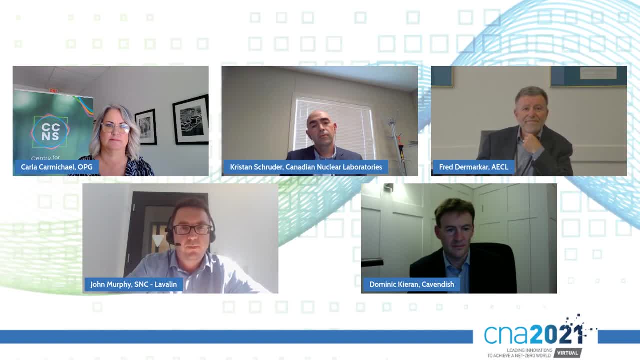 Um, and I think that what we'll also do is, you know, build our, our knowledge portfolio As we step into decommissioning of these reactors over the next kind of five to 10 years And then, if we can look to export that to other geographies whereby the can do reactors will fall into the decommissioning program at a point in time. I think there's opportunities for us there to to leverage that experience, and we can do that in partnership in, you know, in the future. 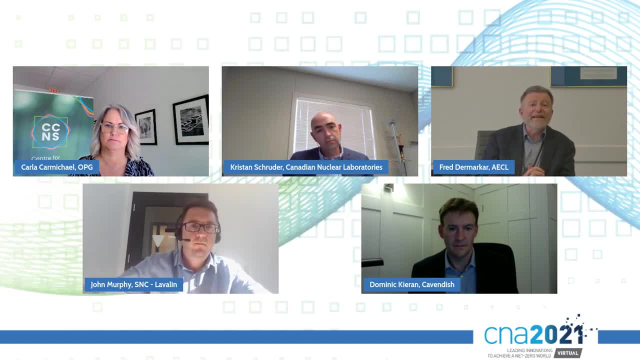 Absolutely. Thanks for that, John And uh Kristen. any last words to Alan, I think uh just just in final thoughts on uh, on this Fred. So in building on uh kind of what people have said right. 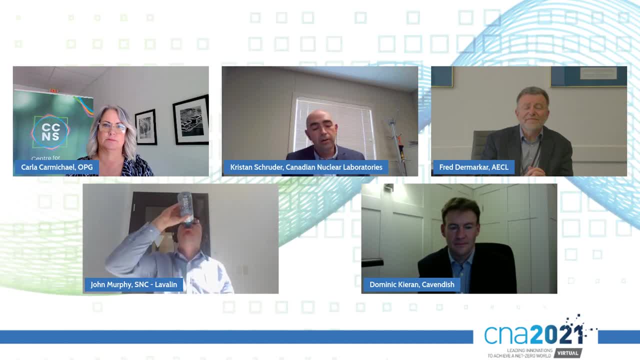 Of collaboration, um, by collaborating, uh with other countries on our decommissioning program. here it's really just building that resume that, um, you know, let's do it safely in Canada, um, with our projects, Uh, and then we can work with our partners to do to bring that outside of Canada and, uh, do some work internationally. 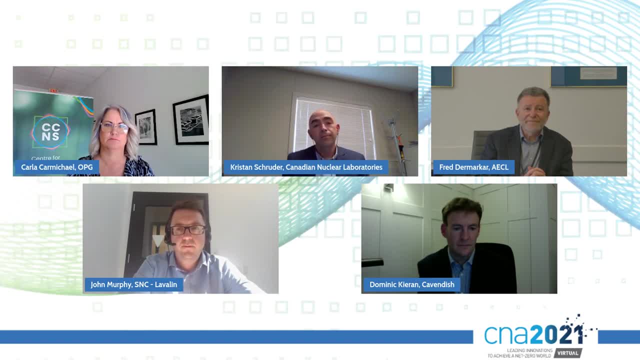 So I think it's about collaborating and demonstrating that we can do it safely here, uh, and then look to do it elsewhere. Absolutely, Uh. demonstrating that we can do it safely here is a great way to end this off, Um, uh. so thanks very much. 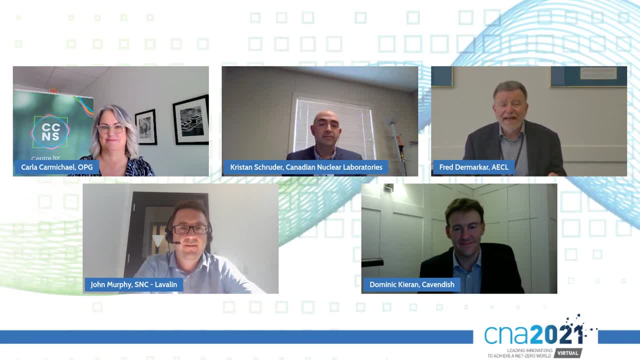 You've been a great panel. It's been a fascinating discussion And, uh, I I want to thank all of you uh, some some great insights shared today. And with that I'll turn it back to the CNA. Thank you, everyone, Thank you.